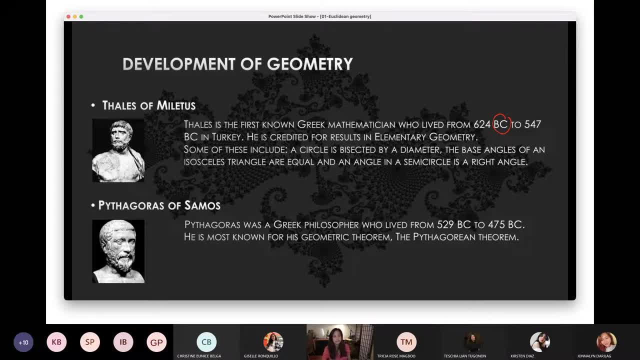 So that's how they're named. So we have here Philz of Thales of Miletus- He's the one who talks about circle that is bisected by a diameter. So we have a circle. it has a diameter- the longest cord that you can put in a circle. 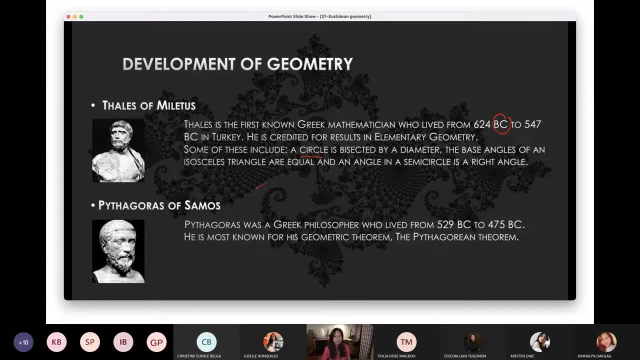 We call it diameter. He also talks about the base of an equilateral triangle. If the two sides of the triangle are equal, then its base, its angles here are equal. And he talks about the angle of a semicircle. If there's half a circle, then if you measure that the angle, there will be 90 degrees. 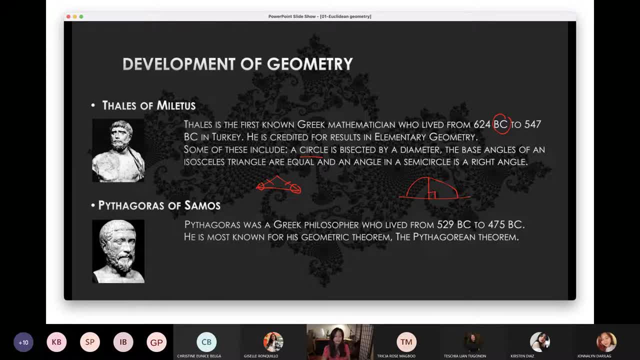 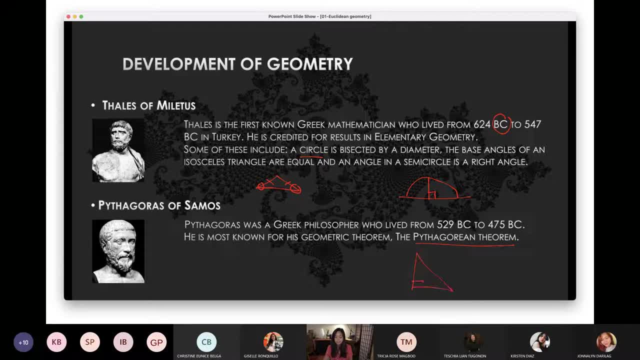 Pythagorean theorem only works with two angles, with right triangles, If you remember. this is the formula: a squared plus b squared is equal to c squared. So yeah, that's Pythagoras where we got the Pythagorean theorem. The next ones are Socrates. 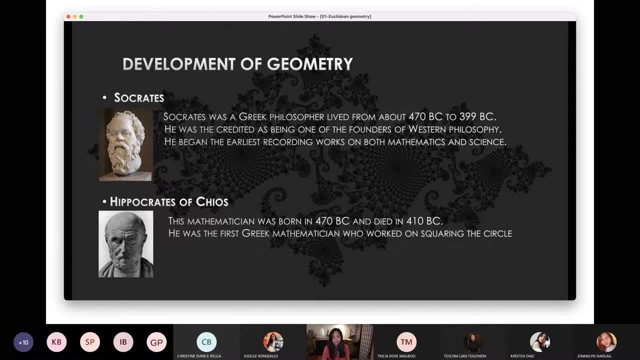 Socrates and Hippocrates. Socrates is very known with his contribution in philosophy and literature, but he actually is a person who has some contribution in mathematics and science, especially in his recordings of his work. So he started that, but of course these are. 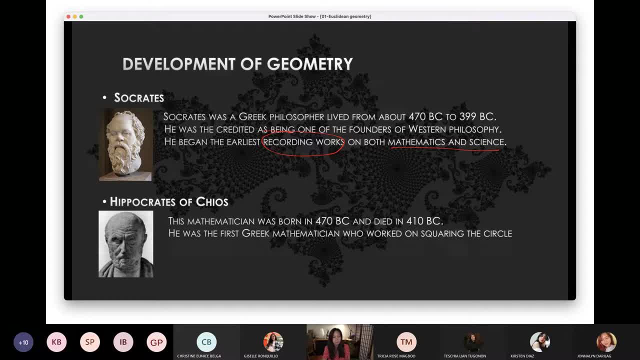 the older people. This is before Christ's mathematician. The next one is Hippocrates. He's the first Greek mathematician. He works with squaring the circles. So, if you remember, the area of a circle is celestial r squared. so why is that squared? so the hypocrisy. hippocrates has something to say with that. the 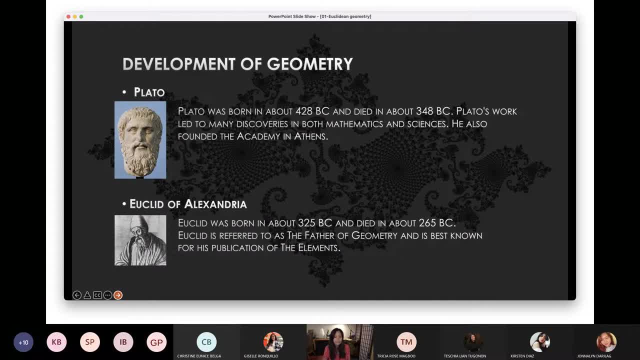 next one is: you're familiar with this, plato. plato is another person who has a high contribution in philosophy and in sciences, in literature, but he, he has he led many works that discovers mathematics and science. uh, discoveries in mathematics and sciences. he led some work that. 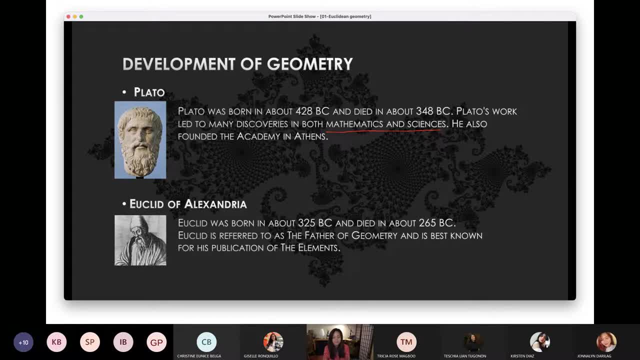 discovers some theories, some concept in mathematics and sciences. he founded the academy of athens. the next one is the guy that we will be talking about today. we call him euclid of alexandria, or simply euclid. euclid is known as the father of geometry. 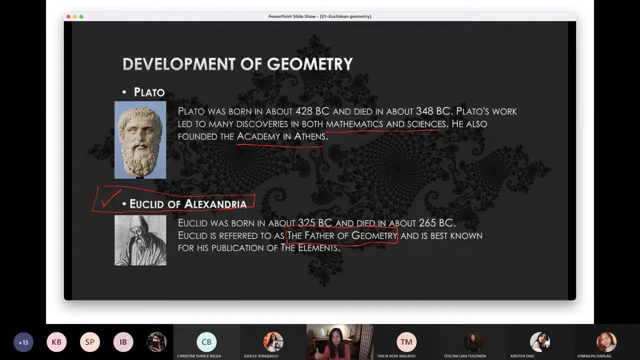 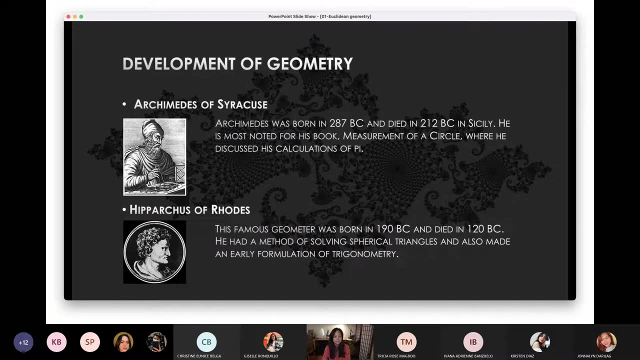 so he's that guy and he's very known with his publication and that is the publication of the elements. the next one is archimedes and hipparchus. so archimedes, he he started. he has a book that talks about the measurement of a circle and how, the, how we calculate pi. 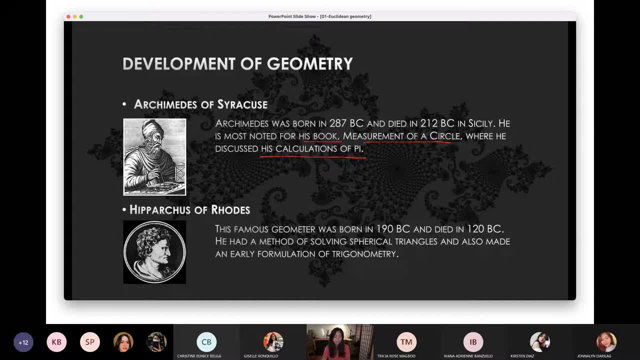 you can learn about the measurement of a circle and how we calculate pi. he is 3.14, approximately, so let's just put approximately 3.14. archimedes has something to say about that a lot and he wrote. he wrote it in a book, hipparchus of. 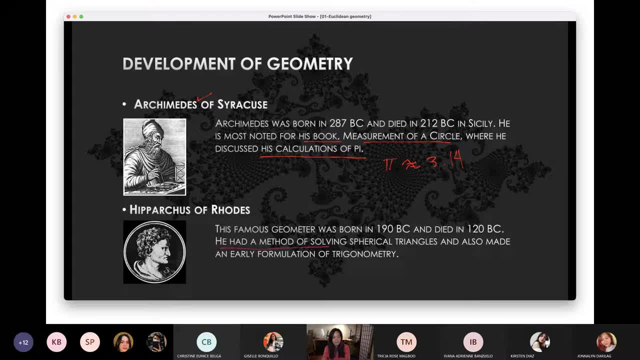 rhodes. he's the one. he had a method of solving spherical triangles and also made an early formulation of trigonometry. if you're familiar- and i think you're familiar- with trigonometry, it's the sine cosine tangent, et cetera, et cetera. 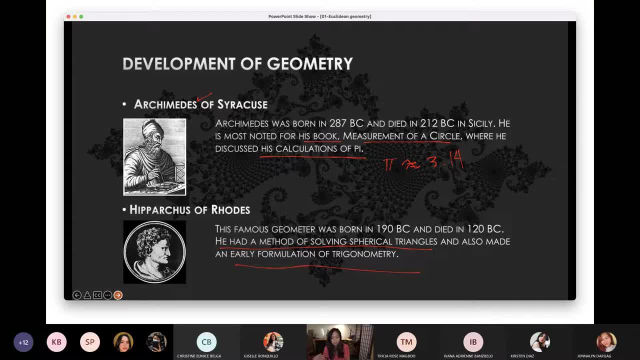 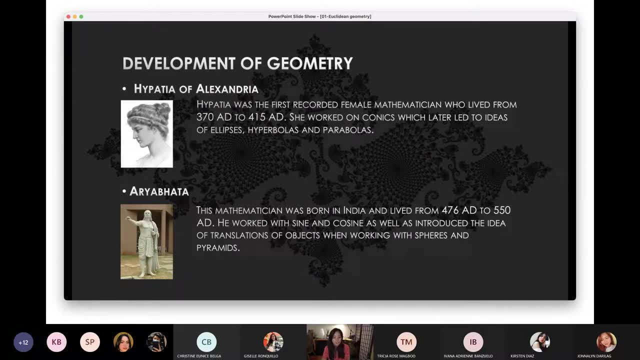 so he started that, but he's not really the one who who coined those concepts, yet he patia, he patia, he worked. she, she's a woman. he, she is a woman who studied in a higher level of geometry that has to do with conics, hyperbolas, ellipses and parabolas. 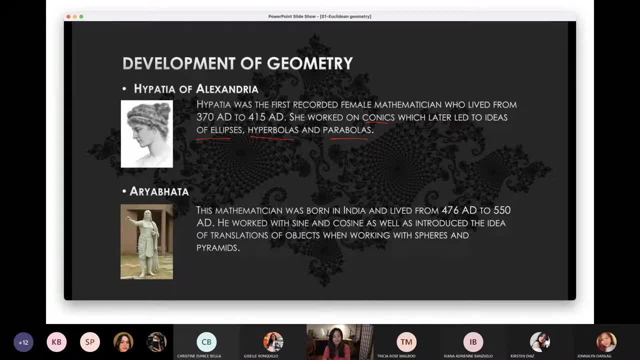 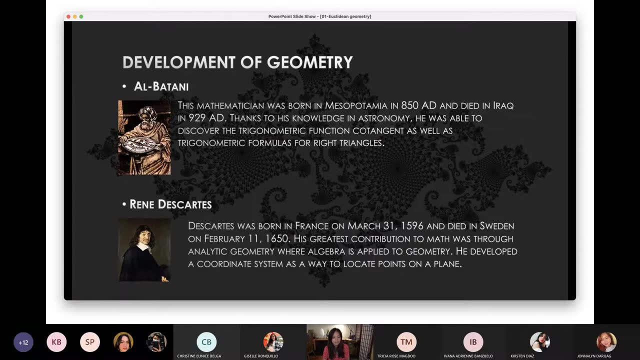 he's from india. this guy has to do work with cosine and sine and introduce some, some ideas that translate from speed with spears and pyramids. the next one is albatani. albatani, it's ad. i know i need to be an ad after wait. 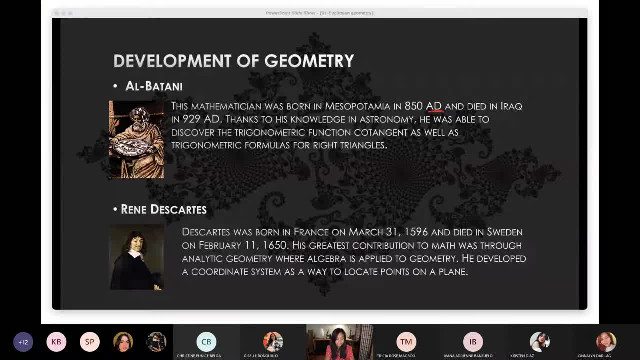 langaisa. ad versus bc. a d means unknown domini in the year of the lord. okay in the year of the lord. okay in the year of the lord in the year of christ. so ad during that time, thanks to his knowledge in astronomy, we were 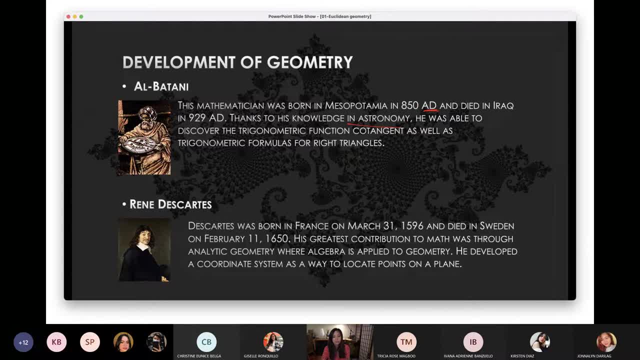 able to discover. he was able to discover the trigonometric functions of contingent- if you're familiar- tangent, cotangent, it's the inverse versa of that- And trigonometric formulas for right triangles. And Rene Descartes. Rene Descartes is a really famous man, Of course, he's after Christ. 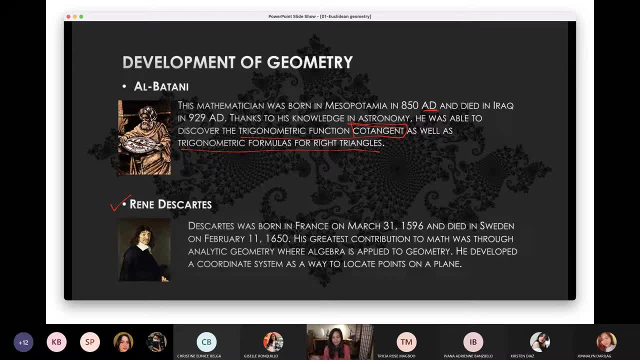 You'll see him in Apiedo, Normally Socrates of Euclid of Alexandria. This is Rene Descartes. Rene Descartes has a lot of contribution in algebra, in mathematics in general and even in logic. If you've noticed before, we have not, and or He has Descartes' rule of sign that can. 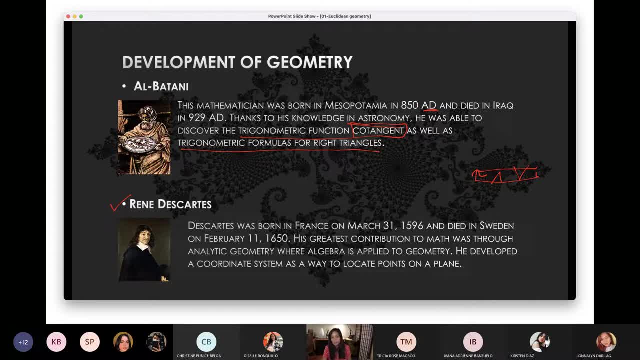 transform that to another form. So Descartes is a very famous mathematician, But he is more known with his coordinate system, the way that we locate points in a plane, And you're going to see that in the next part of this video. 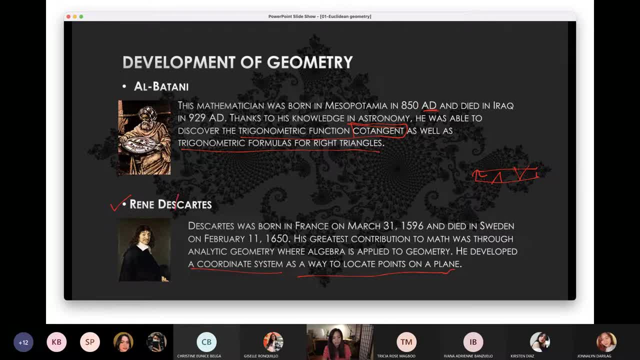 You're very familiar with this. He's the guy who made the partition coordinate system. Yung, X and Y axis, natin, we have X and Y axis. This is the guy who made that standard, the coordinate system. So we have Descartes, the partition coordinate system. 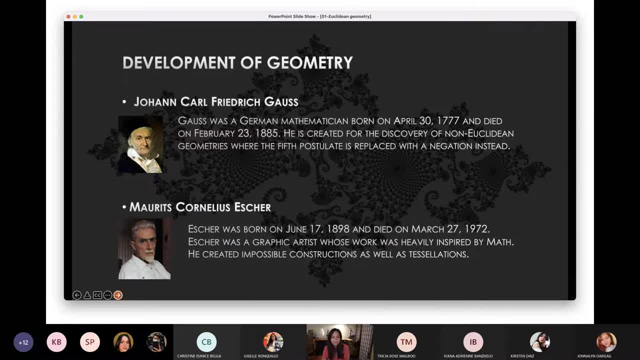 The next one is Johann Carl Friedrich Gauss. He's: He's a mathematician who moved from non-Euclidean geometries. We'll talk about him later. I will show you a video when we say non-Euclidean. Then the next one is Malikius Cornelius Escher. He is not really a mathematician. 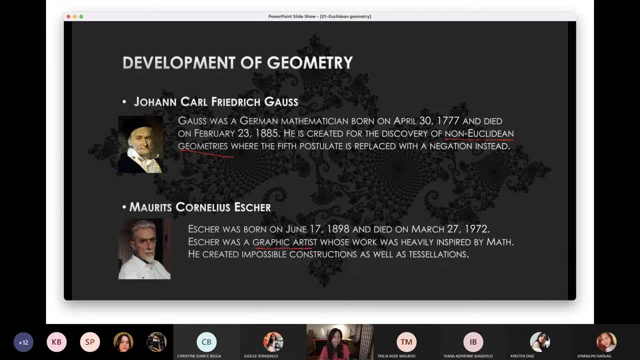 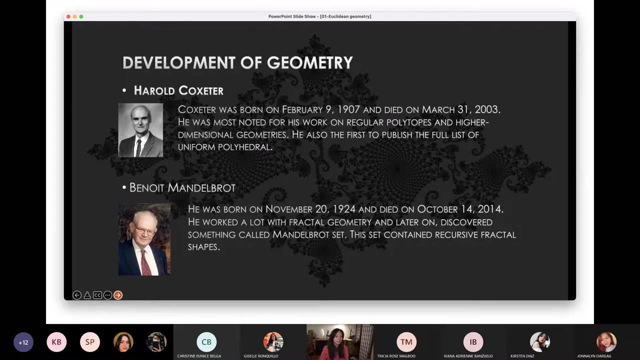 but he's a graphic artist. A graphic artist that heavily inspired by mathematics, So he created impossible construction. So we're not really interested in that. So that's why he's so famous, because he's been working with the most accomplished and intelligent people. 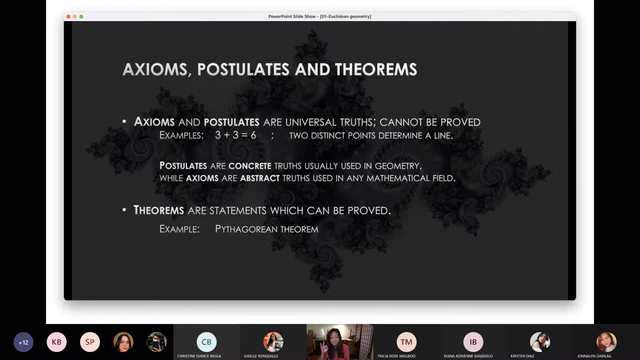 Where's the second one? Where's the third one? Here it is, It's the second one. The third one is Baroque. It's the first one. There are many more, but for geometry they're the basic people in geometry. 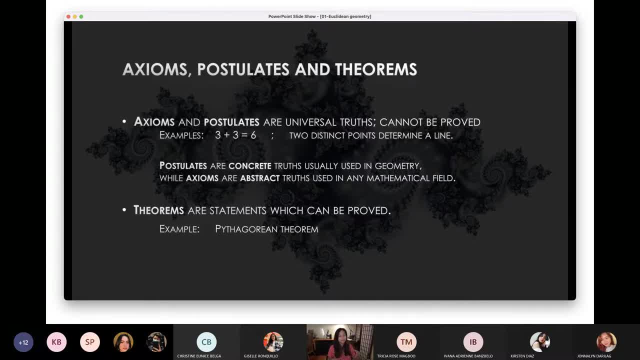 Now let's go to our action, postulate and theorems. So what is the difference between an action, a postulate and a theorem? An action and postulates are called the universal truth. They cannot be proved, but they are true. 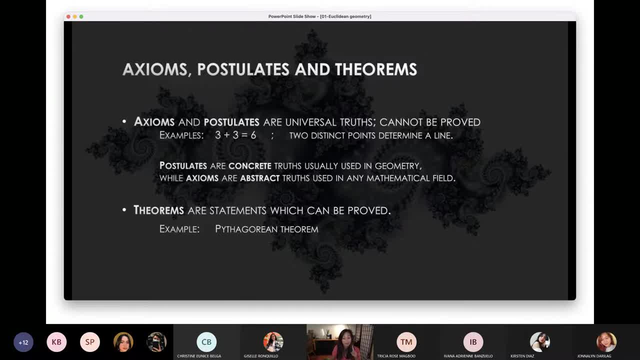 Like let's say: you're beautiful, you're handsome. We cannot prove that, but they're true. Just kidding guys. So we have what we call the action and postulate. You'll notice later why we can say that it's true. 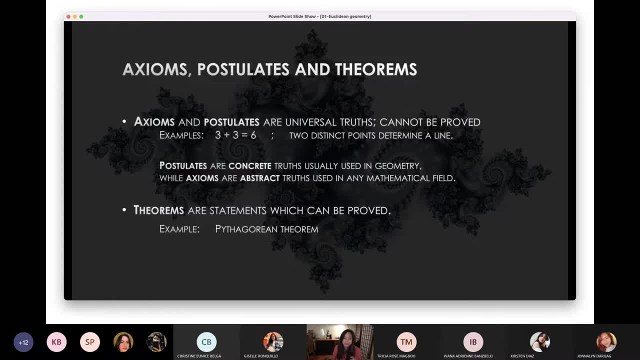 We just can't prove it. The next one is theorems. It's a statement which can be proved. A statement, a theorem can be proved or disproved. So an example of that is a very known Pythagorean theorem: Big Bang Theory. 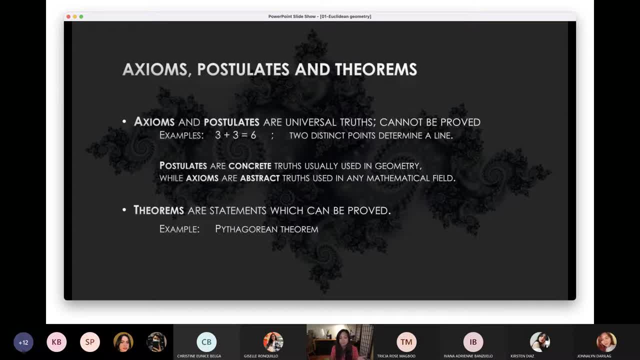 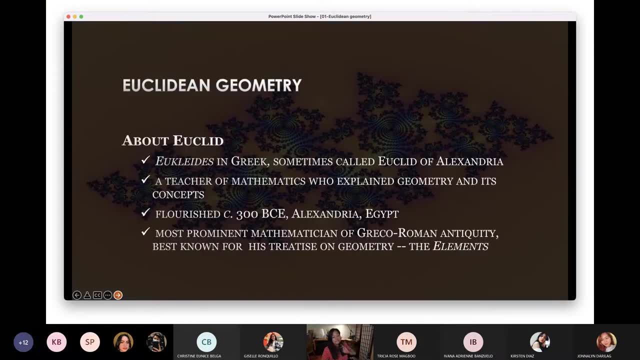 Another. There are theorems that can be proved or disproved with better theorems later on Now. so Euclid, let's go back to the father of geometry, and that is Euclid. We can say Euclid because he actually wrote a book that has the title of The Elements. 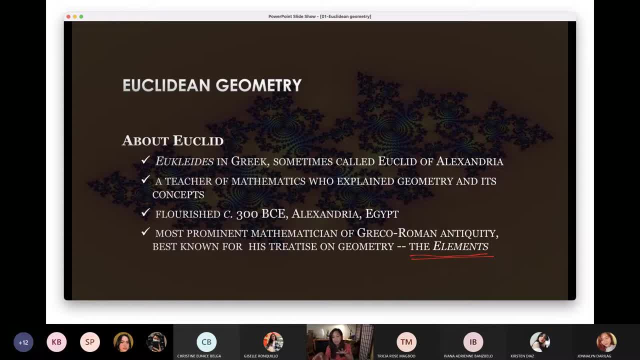 He talks about five postulates when it comes to Euclidean geometry. When we say Euclidean geometry, we are just dealing with what we call a plane-type geometry, our elementary geometry, our high school geometry. So there, I'll read Euclid's definition first. 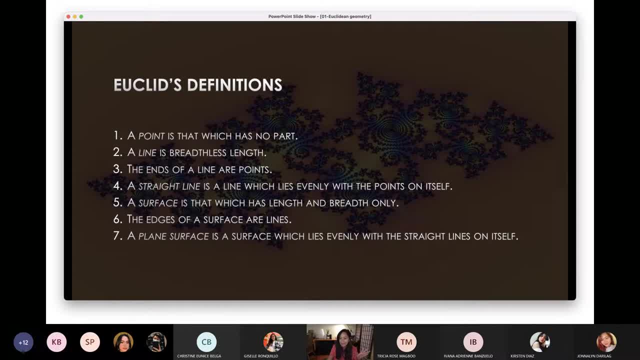 Euclid said before, we wonder if we're different. for example, if I say chair, maybe your definition of chair is different from my chair's definition. So Euclid has this definition so that all of us will think the same. So he said that for him a point has no part. 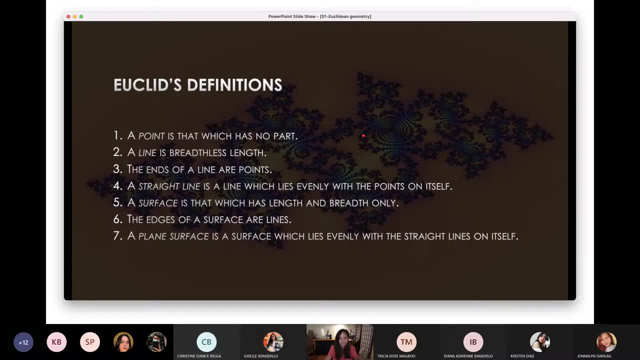 A point has no part. A line has no length. That's a line. The end of a line are points And even within the line are points. There The end of a line is a line, Evenly with points. So if you have a point here, you have a point here, you have a point here. this is a straight line. 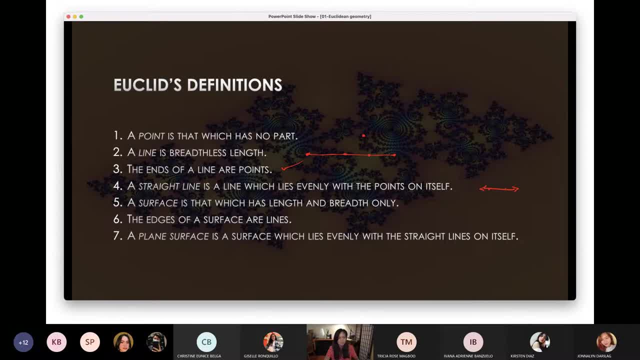 So in a line there are even points. A surface has a length. There The edges of the surface are lines. The edge of this is a line. A plane surface is a surface which lies evenly with straight lines. So let's say I have a straight line here. 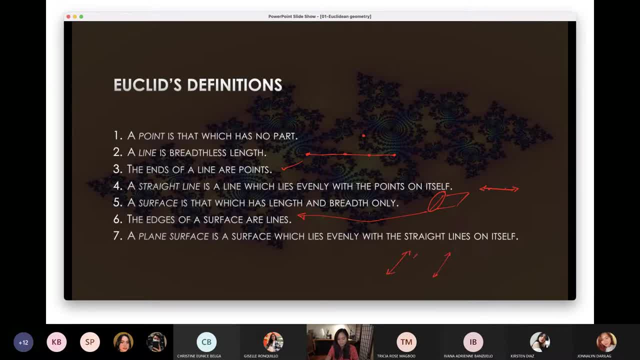 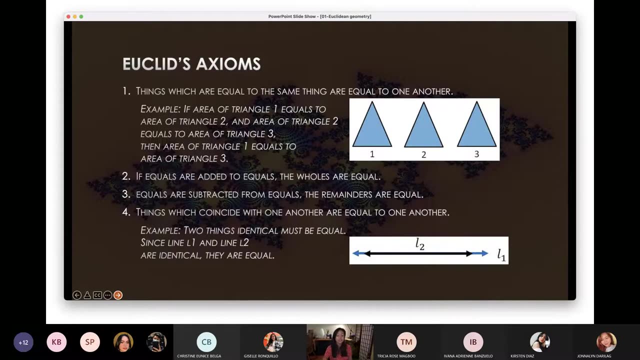 I also have a straight line here. This is a plane. Isn't this a plane? Paper Like a plane. That's what he said. So let's look at the definition of plane, line point, etc. So let's have here Euclid's actions. 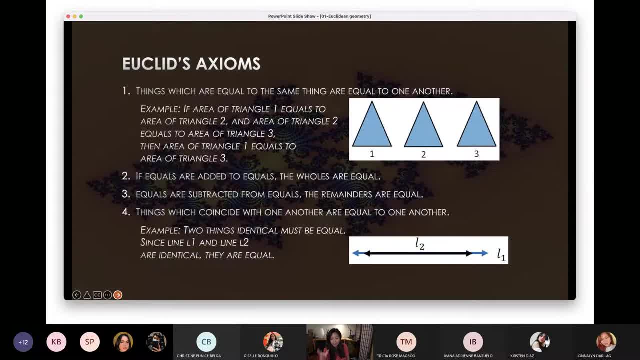 Euclid's actions are very, very obvious And they are obviously true. They're true. So it's like this, Euclid's action number one: Things which are equal to the same thing are equal to one another. It's like this: 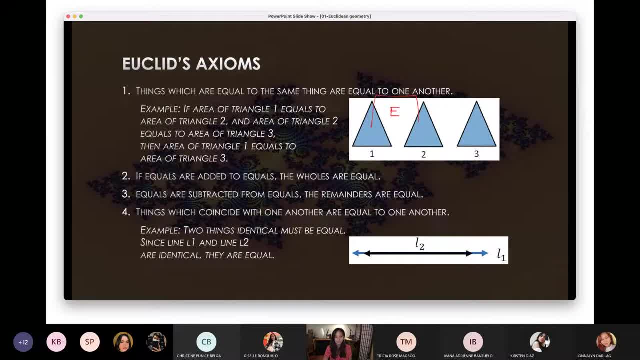 If 1 is equal to 2, and 2 is equal to 3,. therefore 1 and 3 are equal Like duh. they should be equal. But yes, we call that one of Euclid's actions. But this is not the highlight. 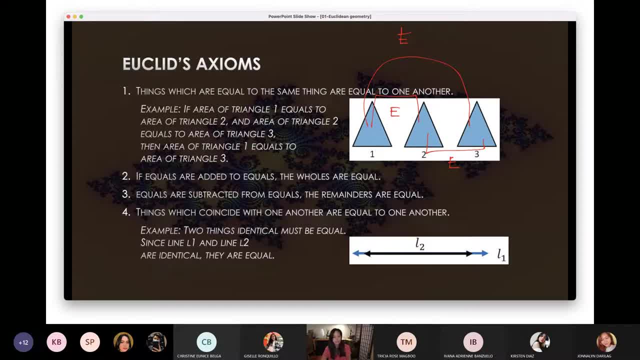 These are just actions. The next one is: if equals are added to equals, the wholes are equal. What do you mean by that? If I have a square, I add a triangle. Let's say: first I have two equal squares, So I have equals. 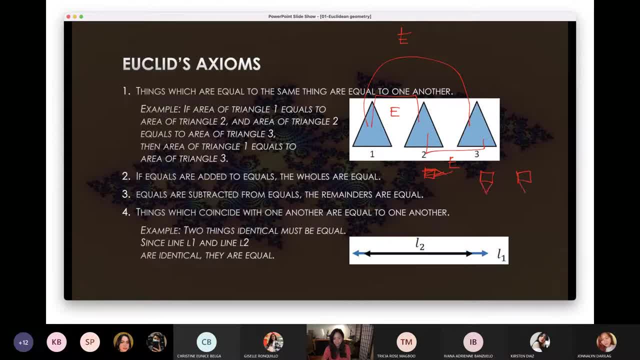 I have two equal squares, I add equal triangles, So I have equals added to. I have equals squares added to equal triangles. The new answers are equal. That's what he's saying. If I have two equals, I add two equals, then those two are equal. 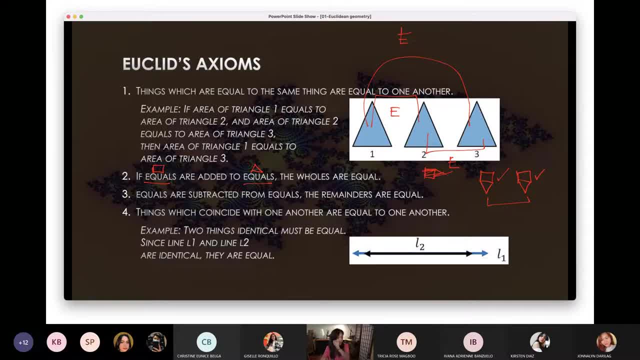 Very obvious. But yes, that's one of his actions. That's why all actions are true. Equals are subtracted from equals. The remainder is equal. So, if you have an equal square, let's reduce it to an equal circle. What's left? the remainders are still equal. 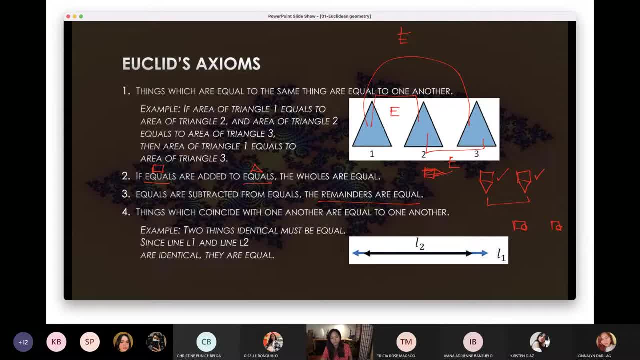 Now, things which coincide with one another are equal to one another. This is a line. Those two lines are equal. If you notice, isn't the black smaller than the blue? Not really, Because they have these ending points, For example, this blue, it will go there forever. 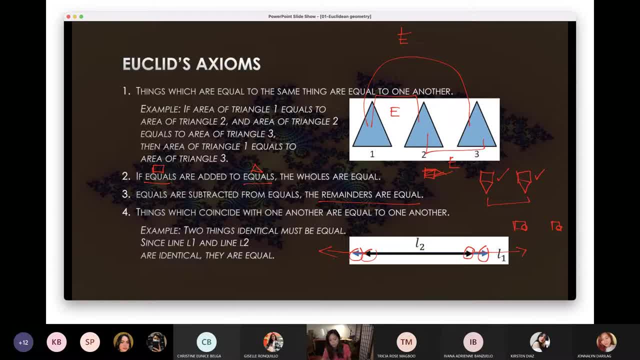 It will extend to the sides. Same goes with the black one: It will extend to the sides. So the two are equal. Now, please remember, the line is different. The line that Euclid is referring to is the line that we know. 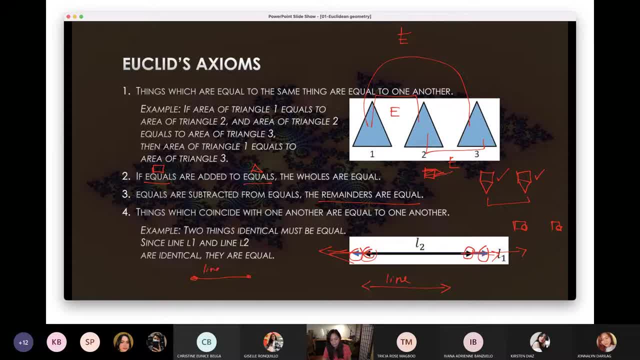 But we are also familiar with the so-called line segment. Euclid calls this a finite line. There is an ending line. That's what he's saying. He calls it an ending line. The next one is: a hole is greater than a square. 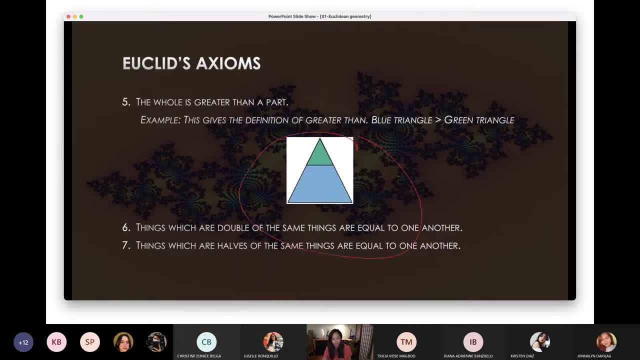 A hole is greater than a part. Of course, if this is your one hole, the small part there and this is your hole, isn't it a hole? It should be bigger than the part. The whole slice of pizza is bigger than the slice of pizza. 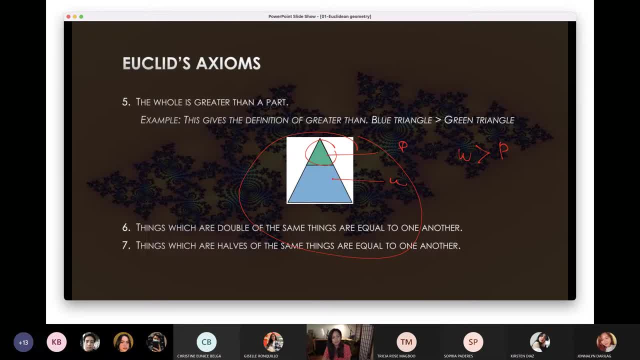 I know it's obvious: Things which are double of the same things are equal to one another. If you have one square, double it. If you have two squares, equal. If you have two squares, double it, They are still equal. 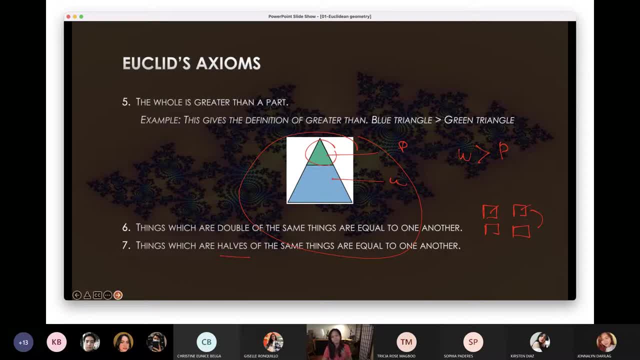 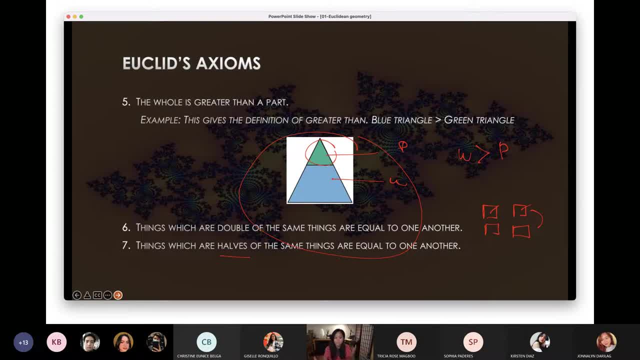 If you have two squares, you will double it. The part is smaller than the whole, etc. These are obviously true, So we call them actions, But this is not the highlight of Euclid's work. The highlight of Euclid's work is this: 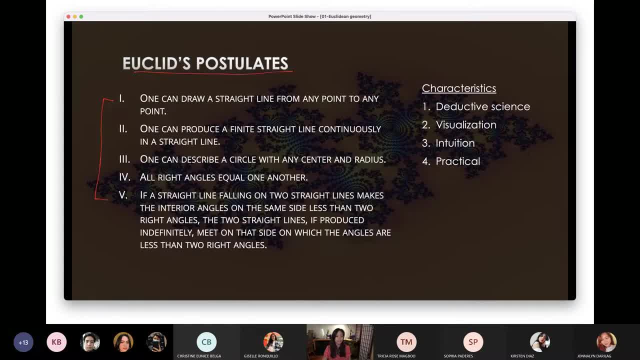 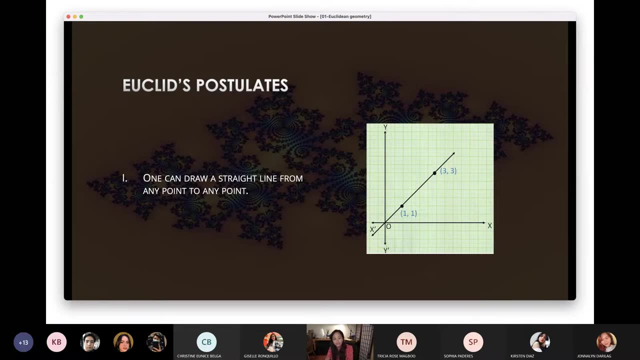 We call them Euclid's postulate. Now, of course, I will just give an overview. There are many points about it, But I will just give an overview. So let's start with the one: Euclid's postulate. One can draw a straight line from any point to any point. 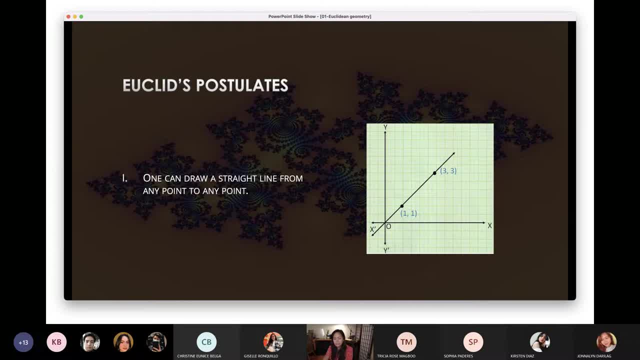 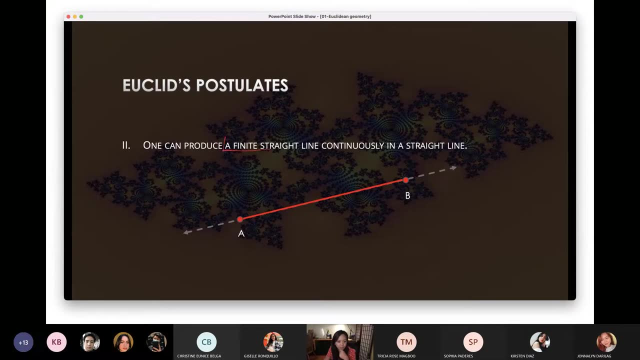 So what you are saying is there are two points. If you have two points, you can draw a straight line. That is what Euclid is saying. If you have two points, you can make a straight line, The next one, One can produce a finite straight line in a straight line. 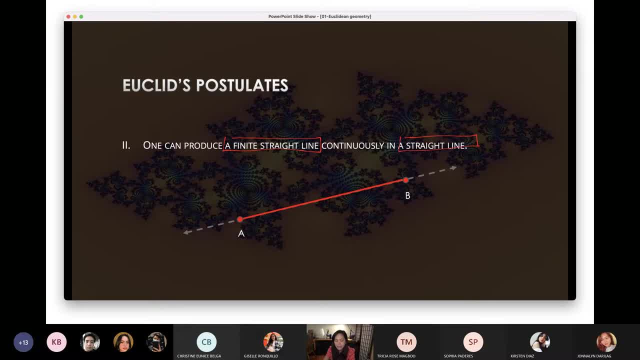 In a continuous straight line. Remember, finite straight line is called the line segment. We are familiar with this. These are the lines that have a segment And this is the line. So, for example, You have a long line, This one. 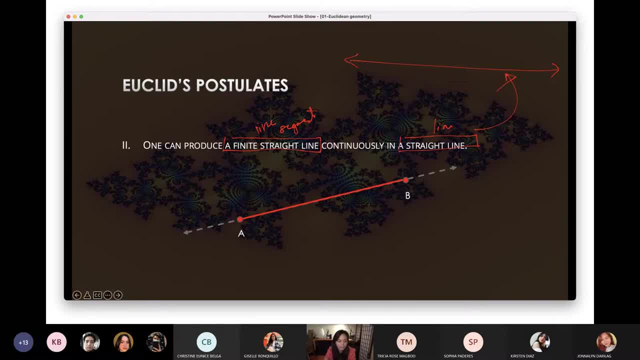 Line, You have a long line, The line segment. You can make a finite segment here. Finite means you have finished. You can make a line segment inside a whole line. So yeah, That's a postulate, That's the second postulate of Euclid's. 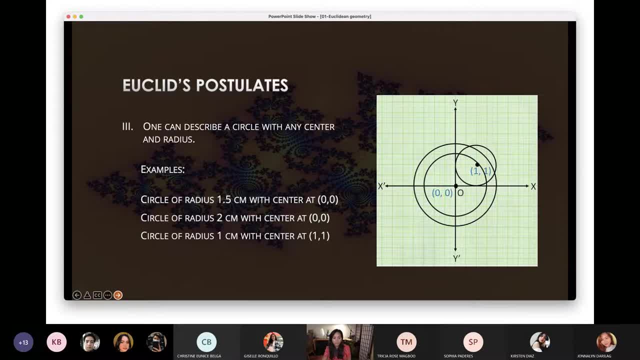 The third postulate of Euclid's postulate. The third postulate of Euclid's has this: One can describe a circle with any center or radius. Euclid is saying: If you have a line, Let's call it a radius. 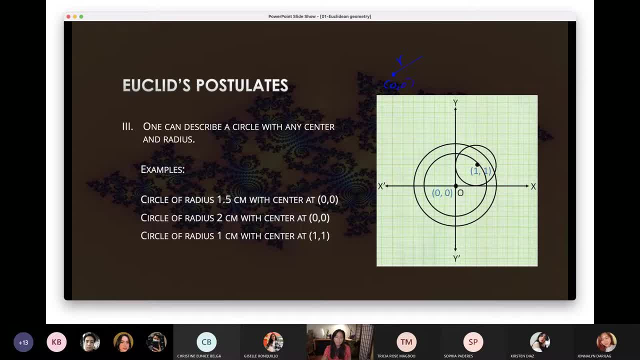 And you have a center. Let's say 0, 0.. You can now describe circles Like this. So, if You can now describe a circle, Isn't that how you would describe a circle If you have a radius And you have a center? 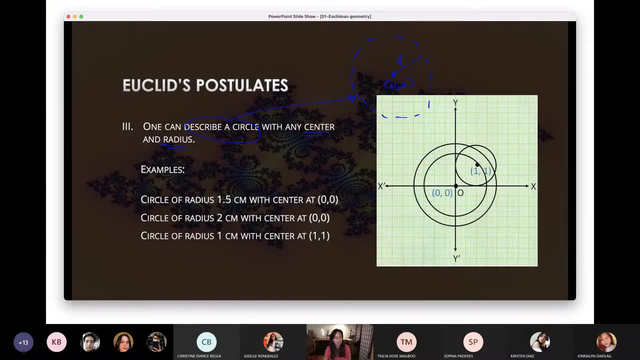 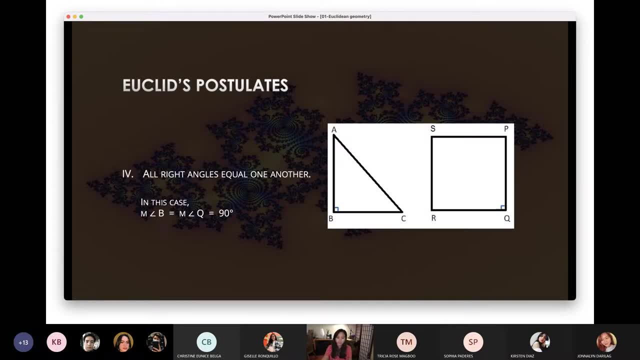 If you only have a circle, That's what it is. And the fourth one Is: all right angles Equal to another right angle, Which is true If you have a Right angle. Right angle. We know that as 90 degrees. 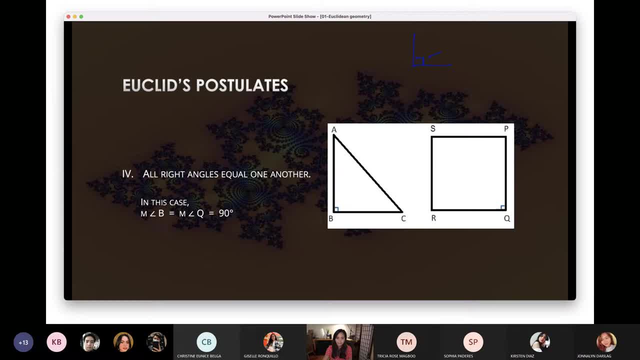 Right, Just like this, Kasi ang right angle mayroon na siyang known like a square: 90 degrees. Sinasabi lang niya na lahat ng right angles, they are equal. Yes, they're equal, and they're equal to 90 degrees. 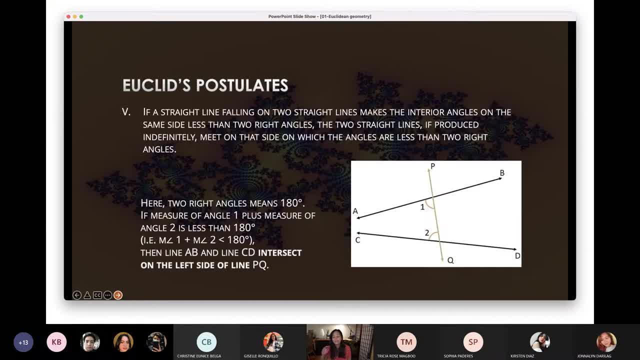 Ganun lang, They're equal to 90 degrees. The next one is the fifth one, So the fifth postulate, ito yung sinasabi nila na medyo debatable. Now, maraming pa to may, maraming concept pa to. 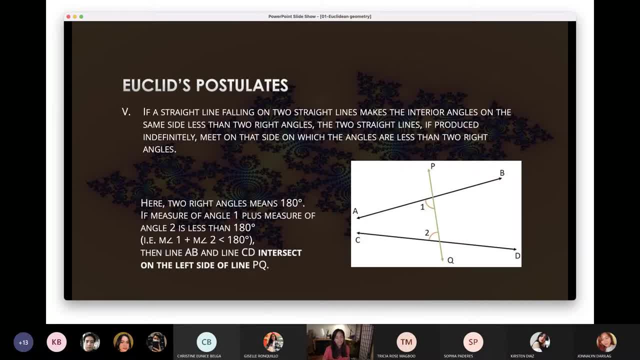 Sinasabi ni Euclid, If a straight line falling in two straight lines makes the interior angle on the same side less than the two right angles. When we say two right angles it's dalawang, 90 degrees, But we're more familiar with the concept of 180 degrees. 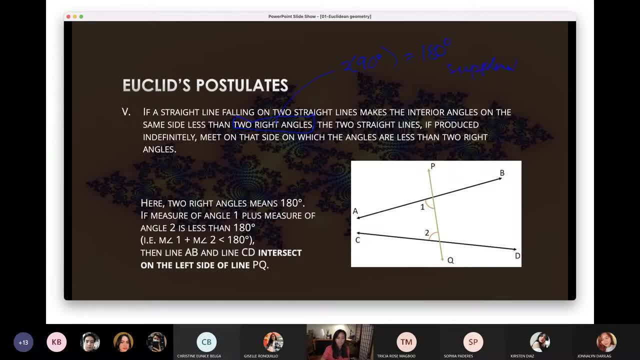 Tinatawag dati ng supplementary. Supplementary angle: 180 degrees. The two straight lines, if produced indefinitely, meet on that side on which the angles are less than the two right angles. Sinasabi lang niya, kung meron kang dalawang line. 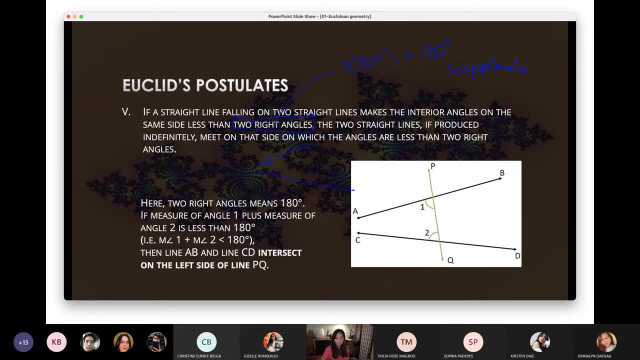 Kung meron kang line na magmimit sila, Magmimit sila may dalawang line, Tapos may isang line na dumaan siya sa gitna. We call it the transversal line. Sabi niya itong, nasa loob daw. 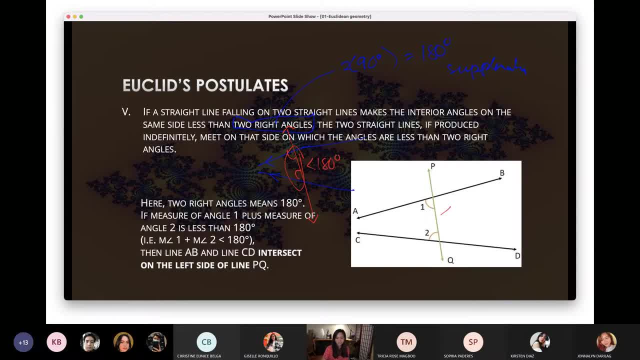 This will be less than 100 degrees. 180 degrees Ayan 180 degrees, Pero kung parallel naman yan, Kung parallel naman yan, Ito, itong dalawang nasa loob, equal naman yan sa 180 degrees. 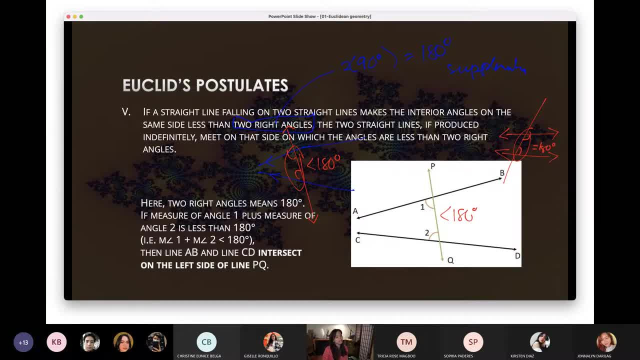 Pero more of ang ginagamit talaga ni Euclid ay, Kung meron kang line At meron kang point dito somewhere here, Sabihin natin may point ka dito, Pwede kang gumawa ng isang parallel line. 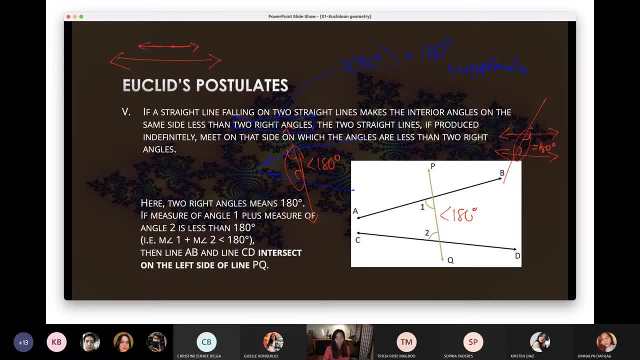 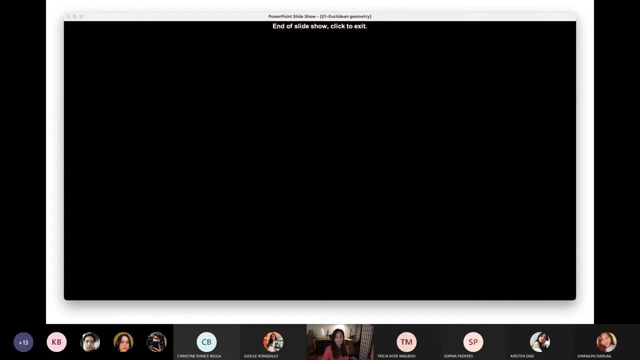 Ka-parallel nito. So pwede ka ding gumawa niya So kasama siya sa 5th postulate ni Euclid. So that's it. That's the Euclidian geometry. Now I will show you another powerpoint. 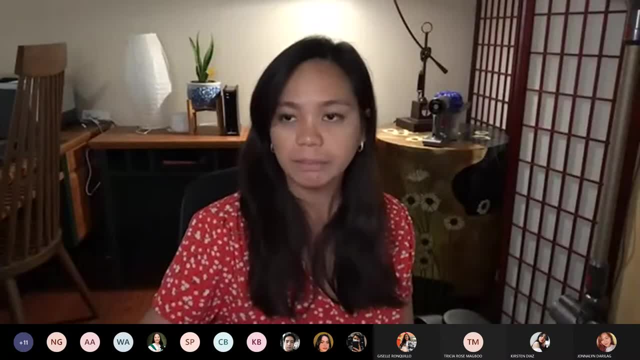 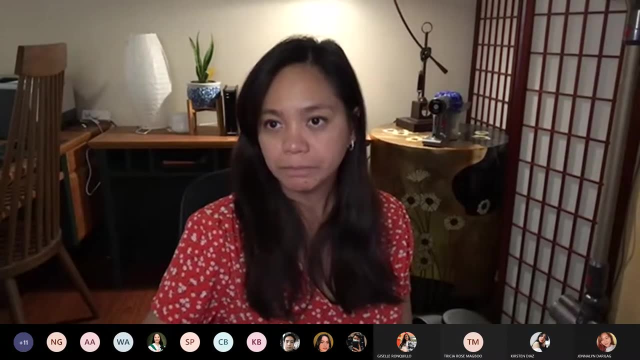 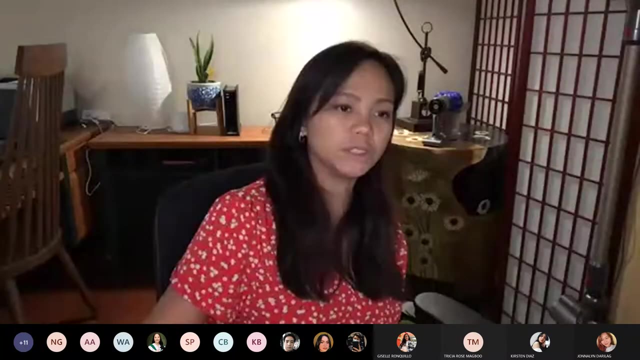 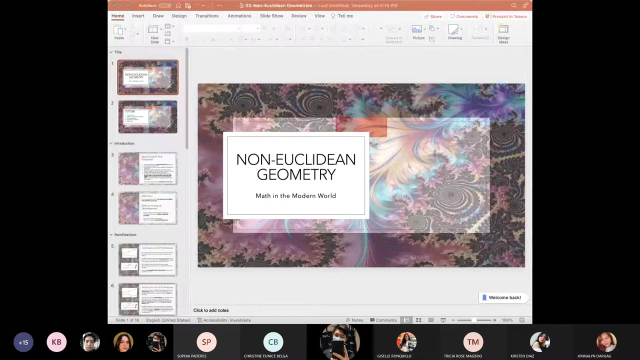 Did I record this already? Yes, I record this already. I will show you another powerpoint. You know that the Euclidean geometry is the one that we had, is the one that is discussed in our elementary and high school days, and even college days. 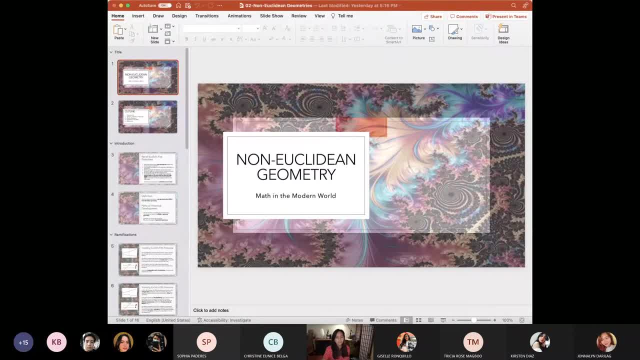 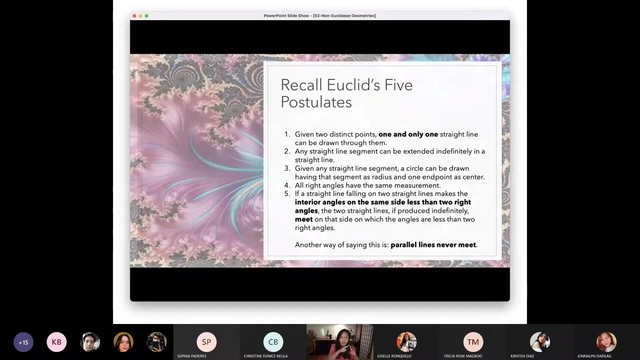 But it's also a concept of non-Euclidean geometry. So in non-Euclidean geometry there are five postulates of Euclidean geometry. If you have two distinct points, you can make one and only one line. We have another one. 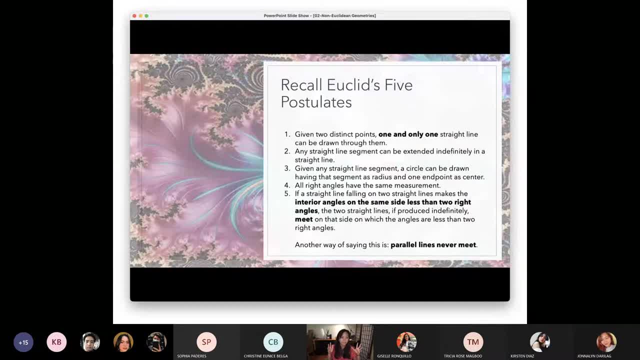 In a straight line segment you can draw a circle. The same measurement And then the fifth one, if it falls into a straight line, makes interior angles on the same line less than two right angles or less than 180 degrees. And then if the two lines- if produced indefinitely- meet on the other side, the angles doesn't do two. 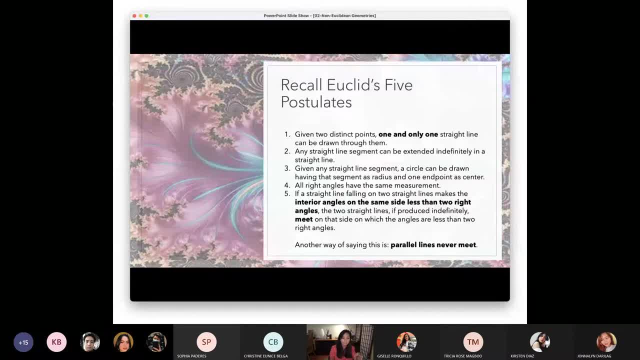 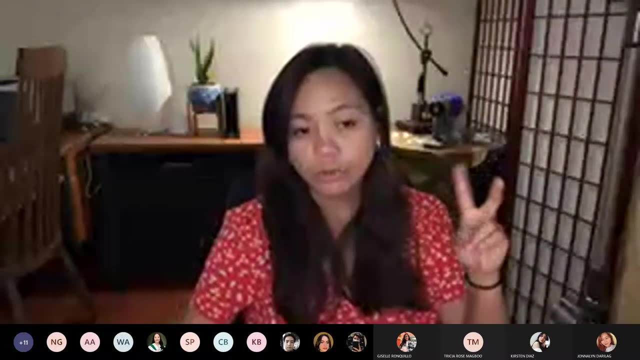 Another way of saying this is: parallel lines never meet. It's not so obvious In this statement, but it's included in the long statement of Euclid. Now I want to discuss the two types of non-Euclidean. There are other non-Euclidean geometry. 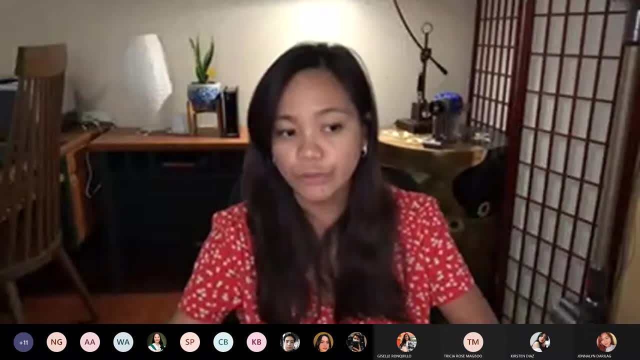 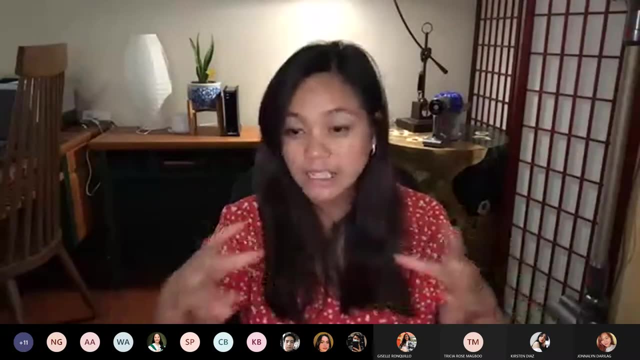 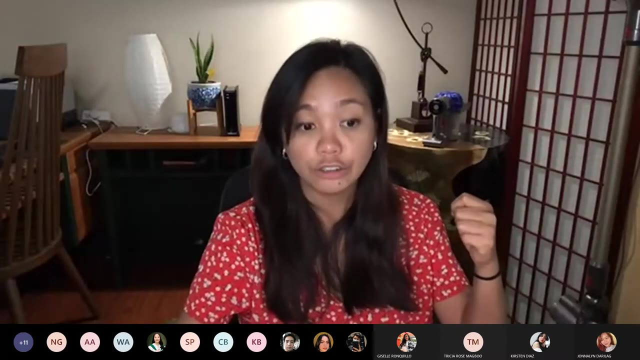 I want to discuss it here, but I think it's better if we watch a video about it, Because it's not two-dimensional, It's not drawing a line, It's not simple, So I will show. I will show you a video about non-Euclidean geometry. 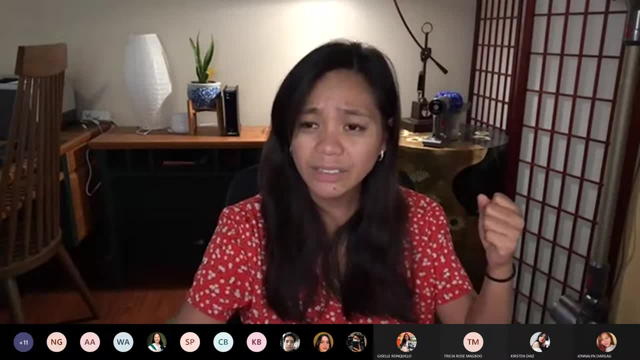 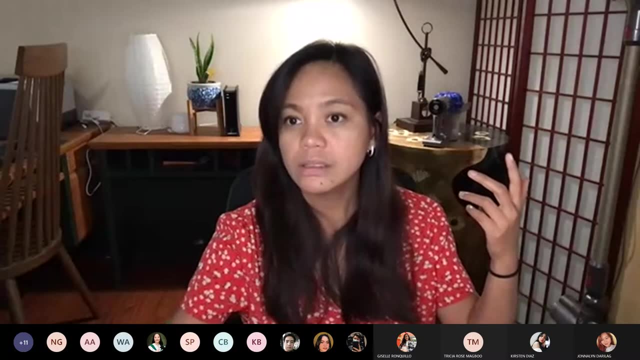 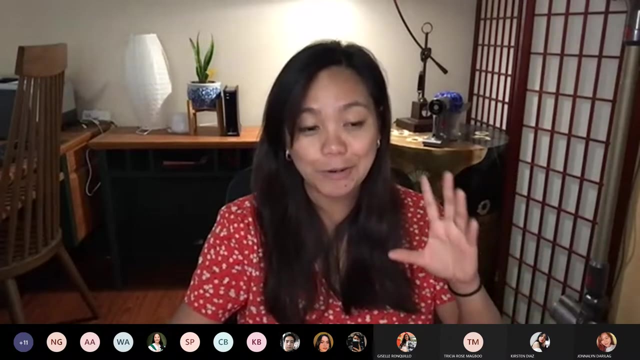 So I got. I think this is the best. I look for better ones, but I think this is the best way to explain non-Euclidean geometry, And you will understand why a video is needed for this. So, guys, can you do this? 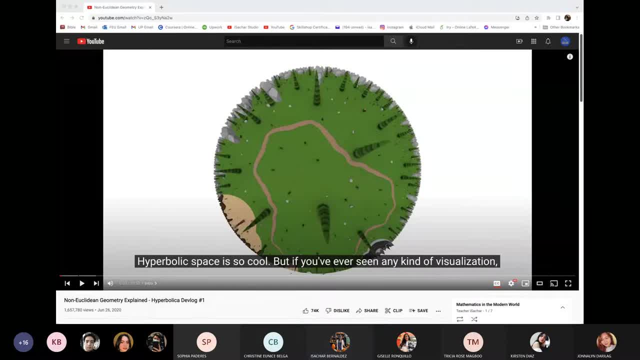 So, guys, can you tell me, if you get it, What kind of visualization? hyperbolic space is so cool, but if you've ever seen any kind of visualization, odds are it was this. this, oh God, the worst one, please. 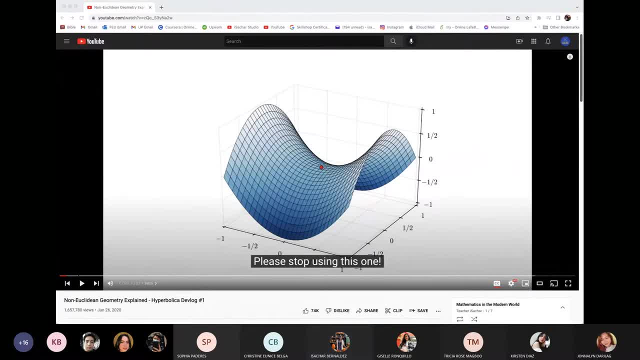 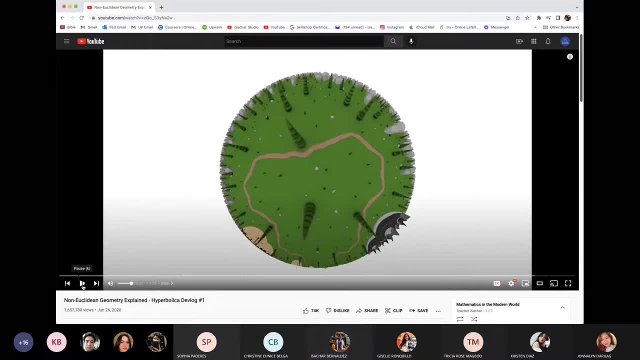 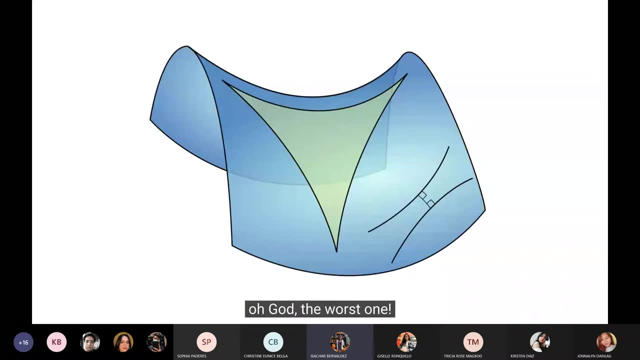 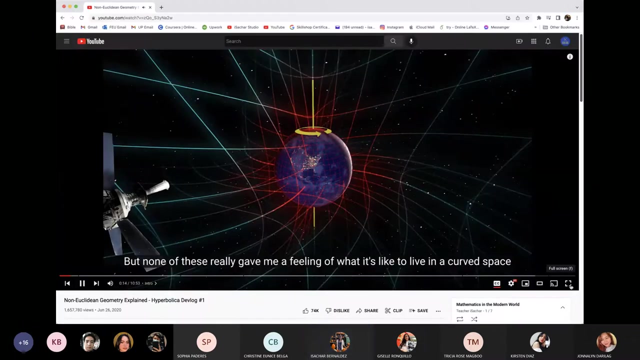 Not even me, John. Yes, Okay, that's good. Okay, I'll, I'll. I'll start that, Thank you. Hyperbolic space is so cool, But if you've ever seen it, If you've ever seen any kind of visualization, odds are it was this or this or, oh God, the worst one. please stop using this one. but none of these really gave me a feeling of what it's like to live in a curved space. 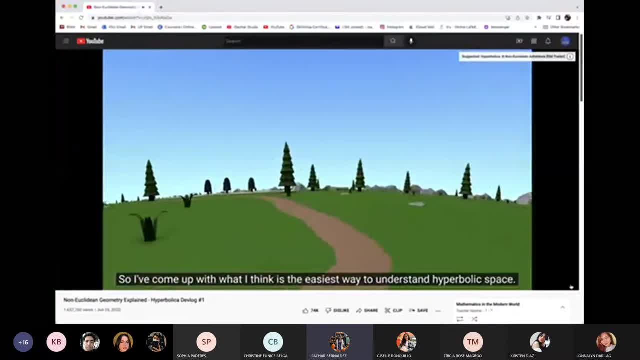 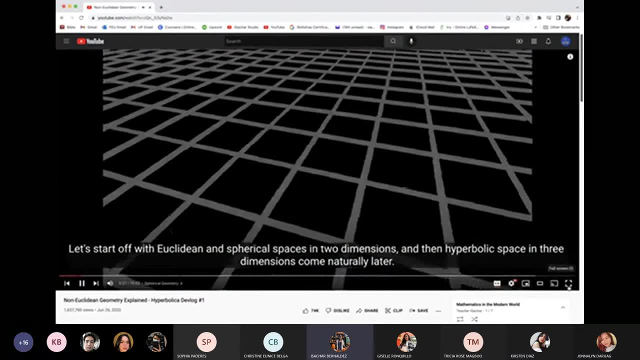 And that was the reason I came up with what I think is the easiest way to understand hyperbolic space. Let's start off with Euclidean and spherical spaces in two dimensions, and then hyperbolic space in three dimensions come naturally later. So here's just a regular flat. 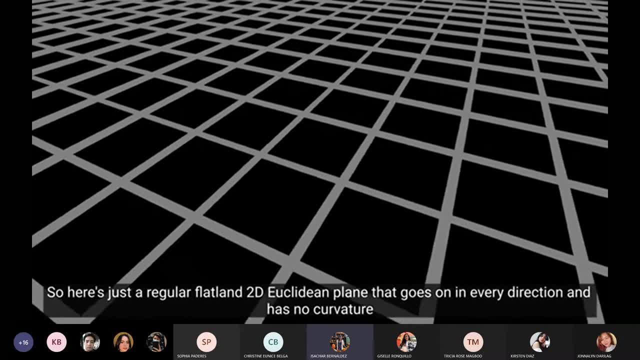 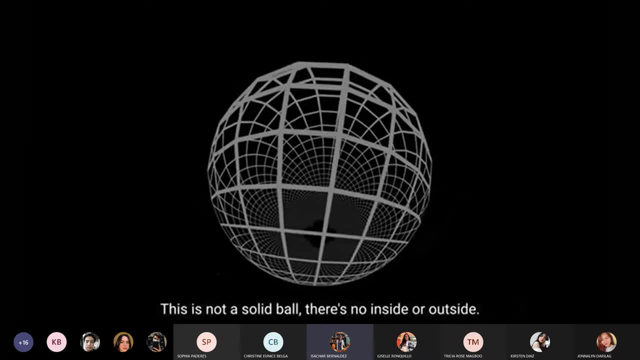 Land 2D Euclidean plane that goes on in every direction and has no curvature. But if we add some positive curvature we get a spherical shell. This is not a solid ball. There's no inside or outside, Just an infinitely thin, two dimensional shell. 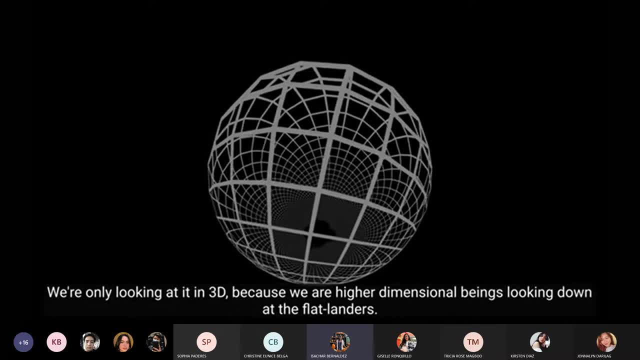 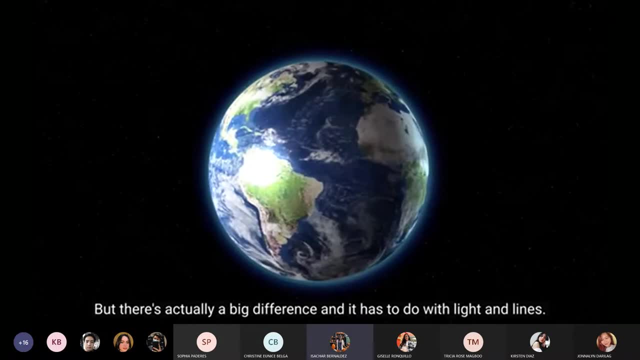 We're only looking at it in 3D because we are higher dimensional beings. looking down at the flat landers, You might think this is really similar to us living on the surface of earth, but there's actually Big. It has to do with light and lines. 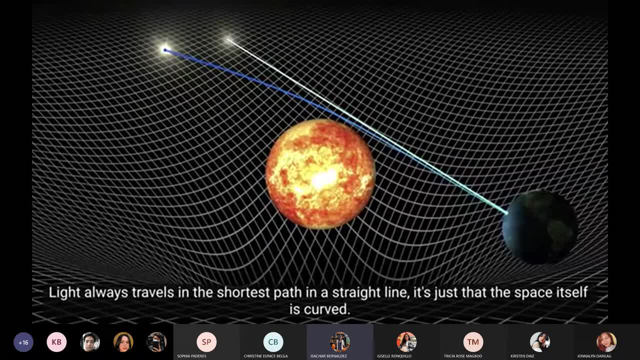 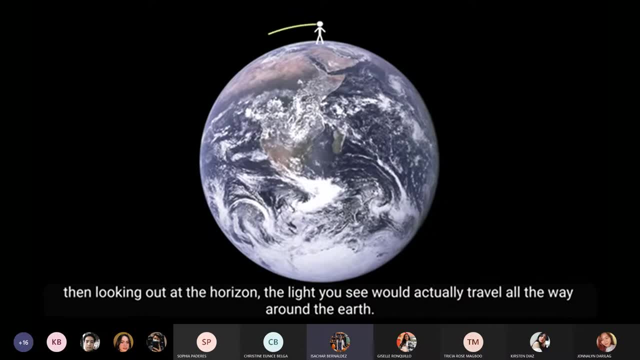 Base of a black light always travels in the shortest path, in a straight line. It's just that the space itself is curved. So if the earth actually had a spherical space time then, looking out at the horizon, flight, you see, would actually travel all the way around the earth. 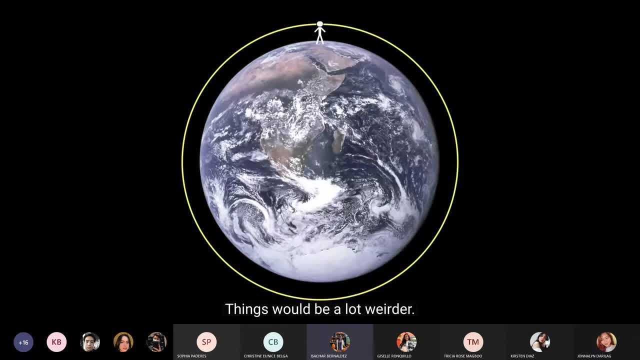 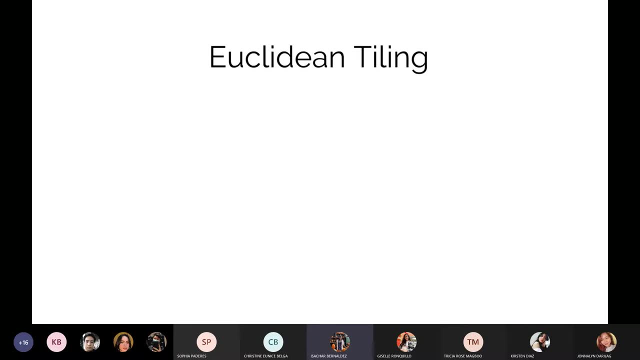 In fact, there wouldn't be a horizon anymore. Things would be a lot weirder. Another way to think about curvature is with tiling. There's only three ways to tile the Euclidean plane: with regular polygon: Four squares at a vertex, six triangles at a vertex or three hexagons at a vertex. 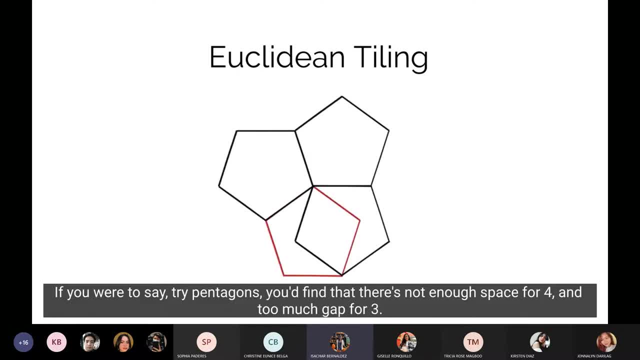 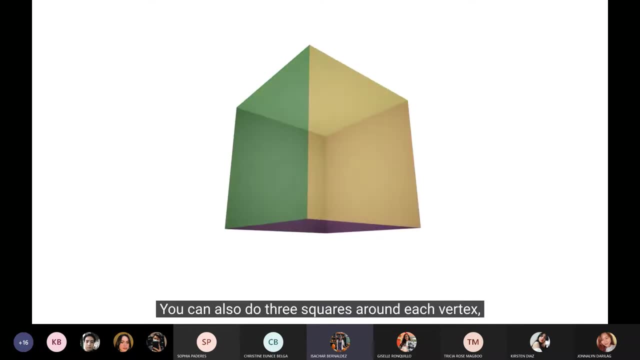 If you were to say, try pentagons, you'd find that there's not enough space for four and too much gap for three. But those gaps could get filled with spherical curvature And you have the familiar dodecahedron. We can also do three squares around each vertex. 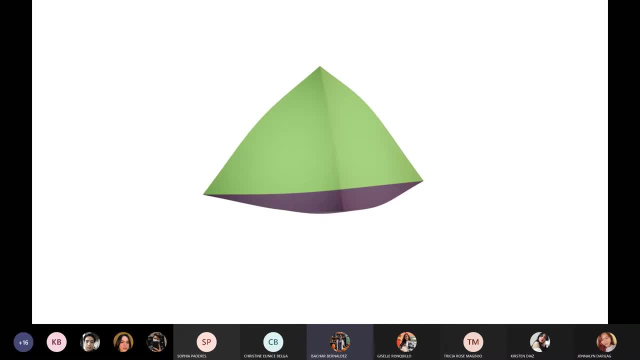 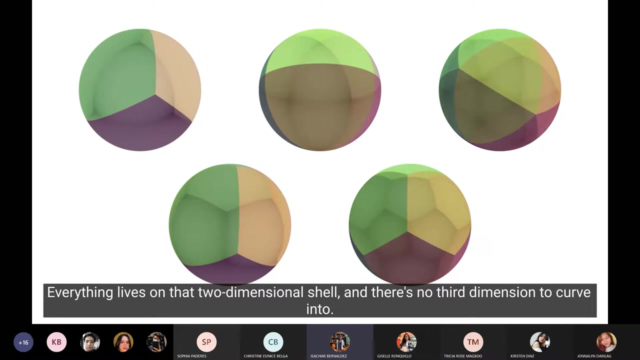 The Three triangles, Four triangles Or five triangles And, just a reminder, all these edges are straight lines. Everything lives on that two dimensional shell and there's no third dimension to curve into. We're only using it to help visualize the space. 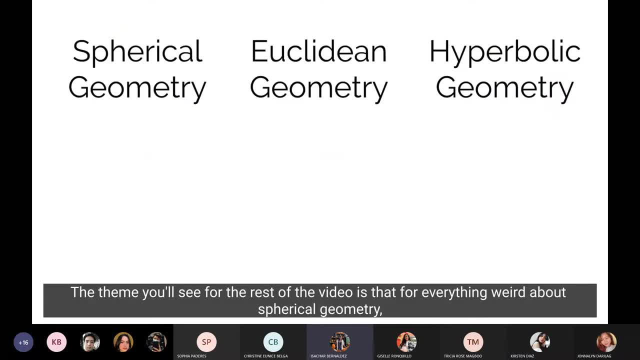 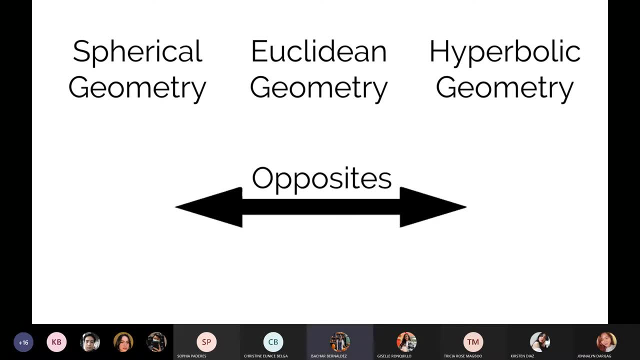 So now let's move on to hyperbolic space. The thing you'll see for the rest of the video is that, for everything weird about spherical geometry, the opposite is true. For example, you just saw that we could have fewer squares around each vertex compared to Euclidean space. 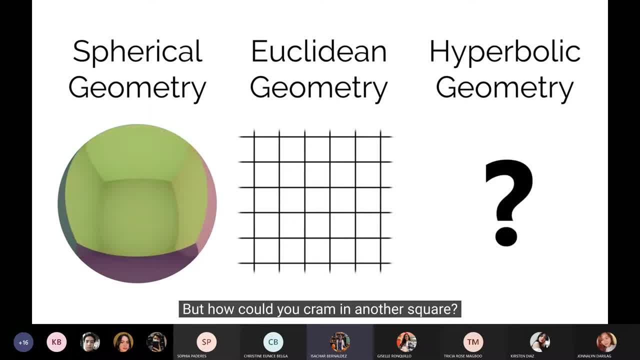 So in hyperbolic space we can have more. But how could you cram in another square? Well, maybe we can do the same trick as the sphere and just bring it out into the third dimension. We can, and here's how it looks. 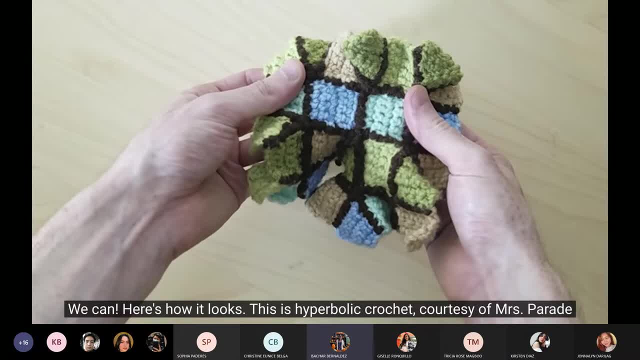 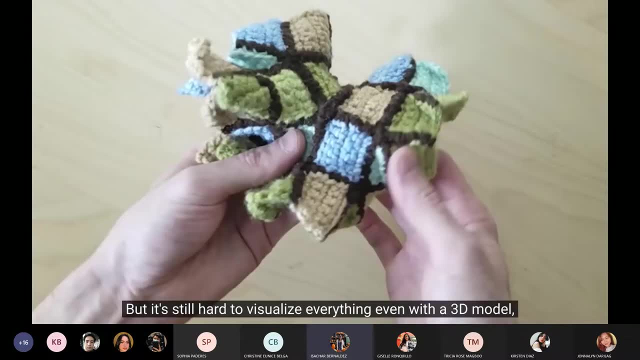 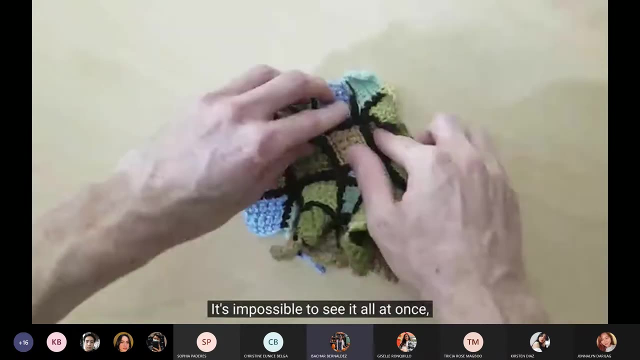 This is hyperbolic crochet, courtesy of Mrs Parade. You can see how five squares meet at every vertex. No, but it's still hard to visualize every Everywhere. It's impossible to see it all at once and it gets even worse as we look at bigger. 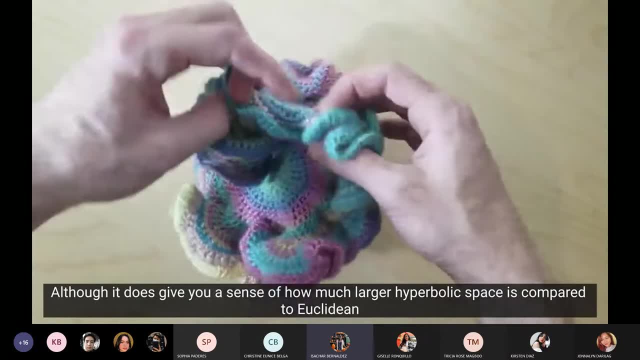 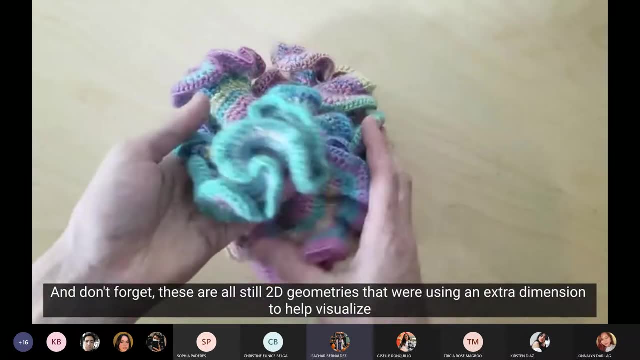 Bigger pieces of the hyperbolic plane, though it does give you a sense of how much larger hyperbolic spaces compared to Euclidean. And don't forget These are all still two dimensional geometries that we're using an extra dimension to help visualize. 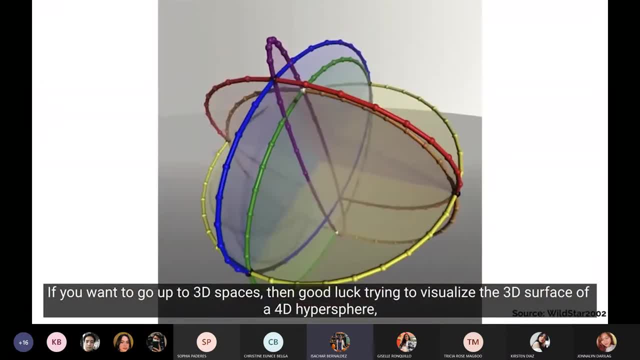 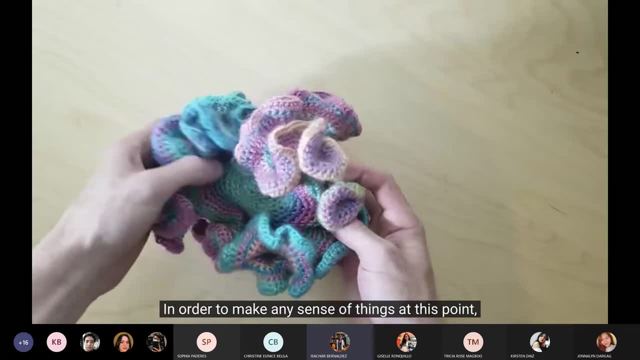 If we want to go up to 3D spaces, then good luck trying to visualize the 3D surface of a 40 hypersphere, or whatever this mess would look like, in four dimensions. In order to make any sense of things at this point, we're going to need a different way to visualize the hyperbolic plane. 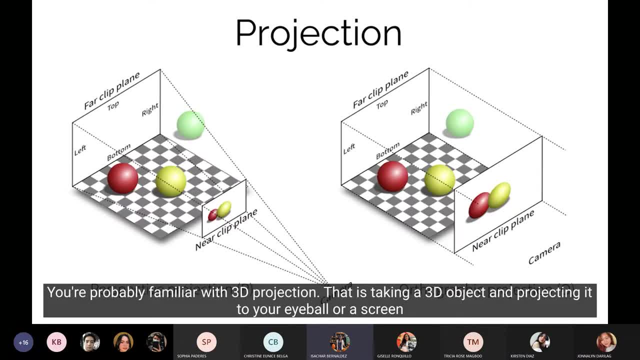 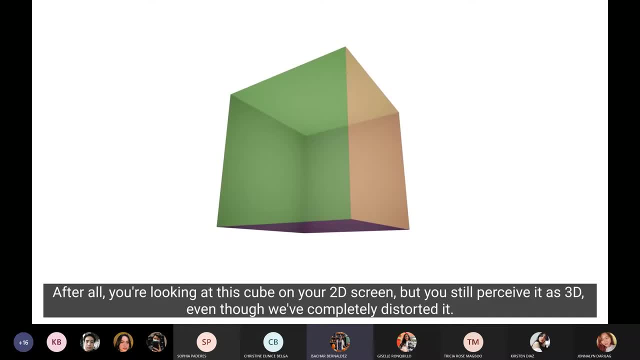 The trick we're going to use is projection. You're probably familiar with 3D projection. That is, taking a 3D object and projecting it to your object, Or projecting it to your eyeball or a screen. After all, you're looking at this key. 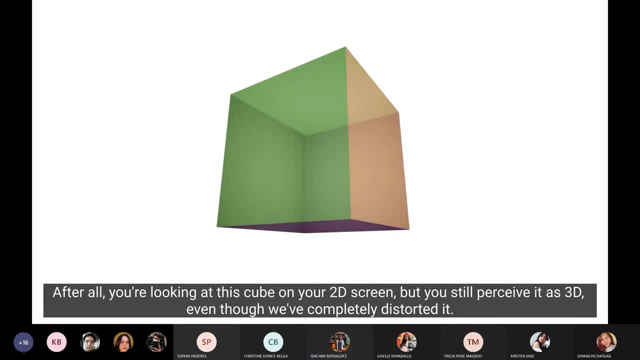 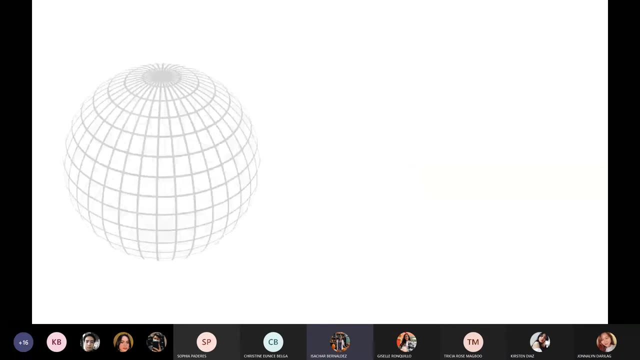 You're still perceiving it as distorted. This is supposed to be a square? Of course not. It's just that projected angles and distances can change depending on where you look at it from and what projection you use. Similarly, we can project a curved geometry to a flat one, or vice versa. 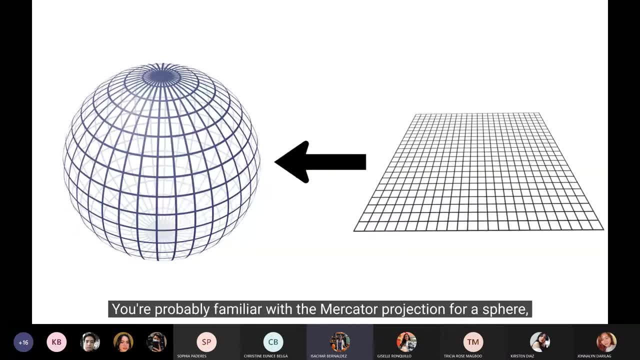 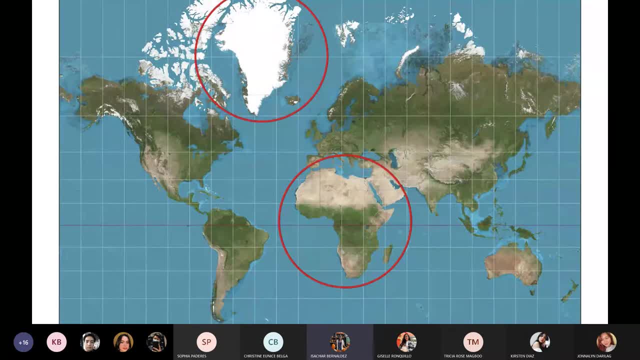 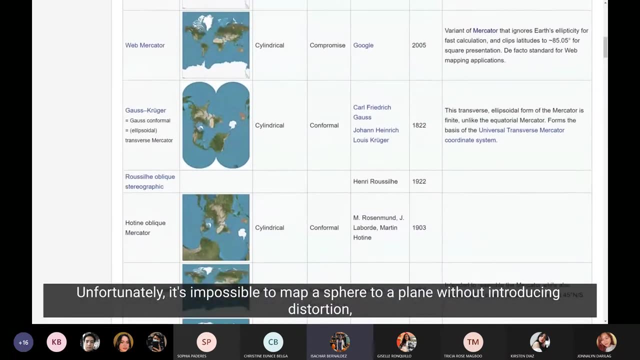 You're probably familiar with the Mercator projection for a second, But, as you can tell, it introduces distortions. Greenland and Africa look about the same size here, but Africa is actually 14 times larger. Unfortunately, it's impossible to map a sphere to a plane without introducing distortion. 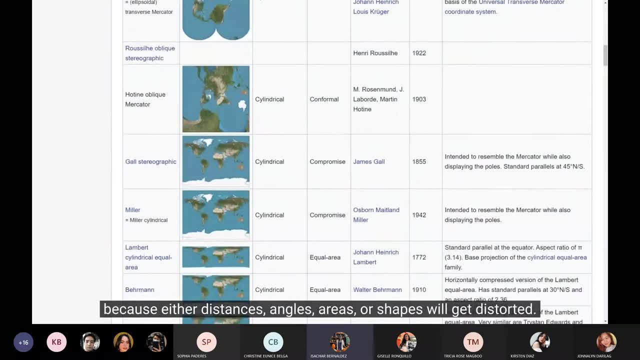 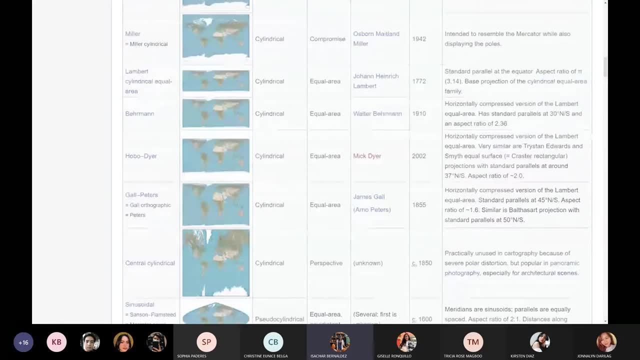 And that's why there's hundreds of different projections, Because either distances, angles, areas or shapes will get distorted, And which compromise you want depends on the application. I'm going to be focusing on a very useful type of projection: Stereographic projection. 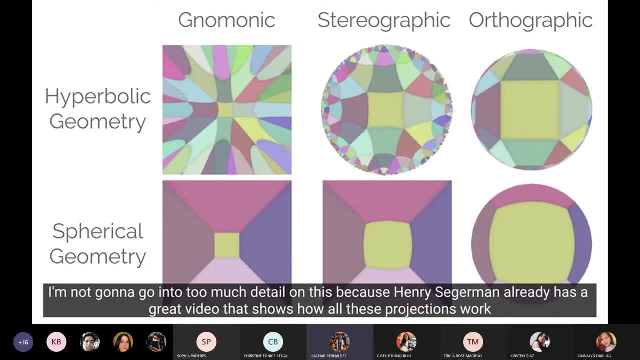 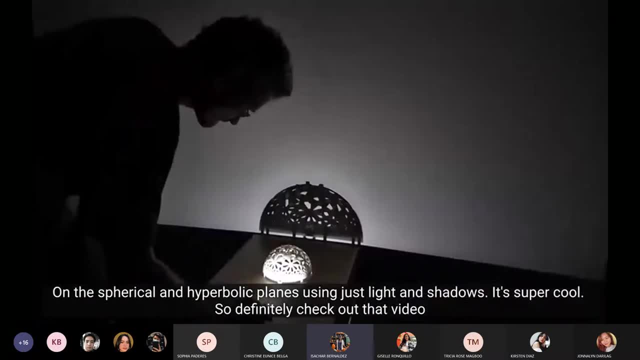 I'm not going to go into too much detail on this, Because Henry Segerman already has a great video that shows how all these projections work on the spherical and hyperbolic planes, using just light and shadows. It's super cool, so definitely check out that video. 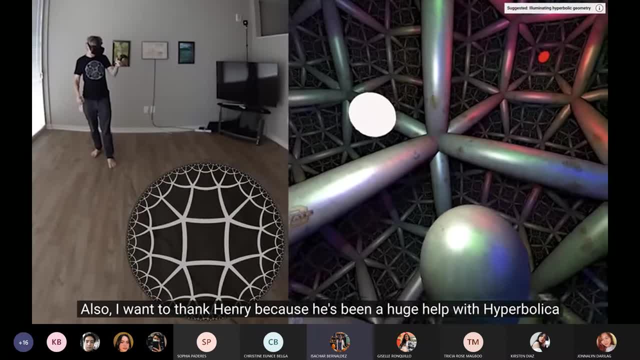 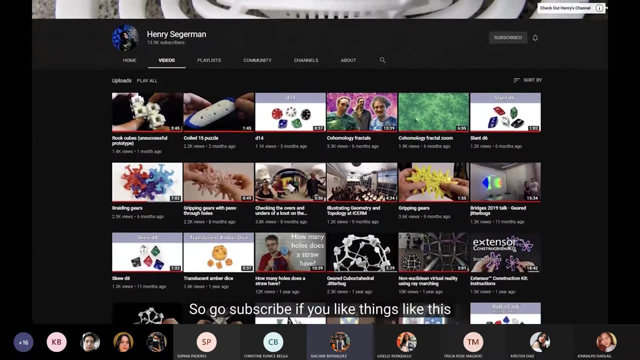 Also I want to thank Henry. Also I want to thank Henry Because he's been a huge help with Hyperbolica. I really don't think I could have done it without him, And his YouTube channel is totally underrated. So go subscribe if you like things like this. 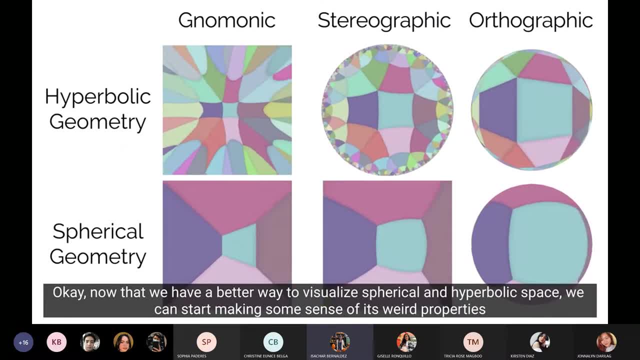 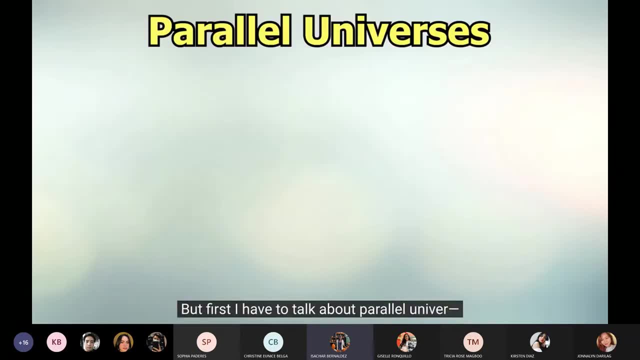 Okay, now that we have a better way to visualize spherical and hyperbolic space, we can start making some sense of its weird properties. But first I have to talk about parallel universe- I mean lines, Parallel lines. They don't exist in spherical space. 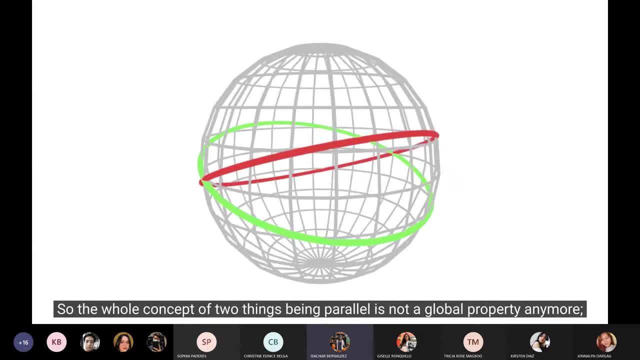 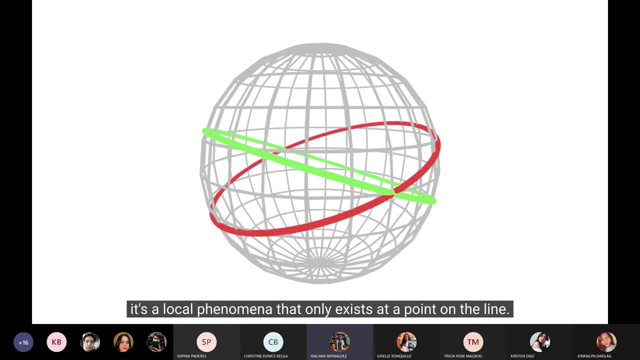 Any pair of straight lines will always converge and intersect eventually. So the whole concept of two things being parallel is not a global property anymore. It's a local phenomenon that only exists at a point on the line. And remember how everything hyperbolic is the opposite of spherical. 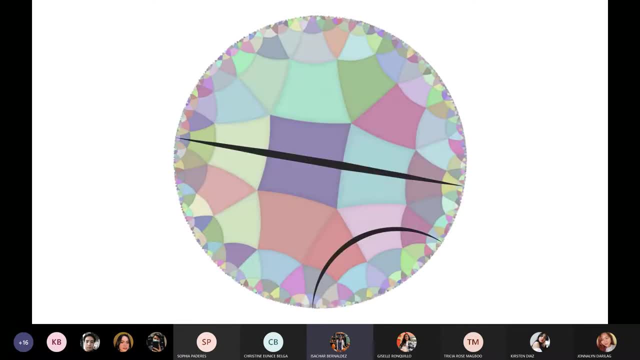 Well, in hyperbolic space, lines will always diverge. Remember, both of these are straight lines, Just like how. this is actually a square. It just depends on what angle you're looking at it from. So walking over to the other line will shift the perspective. 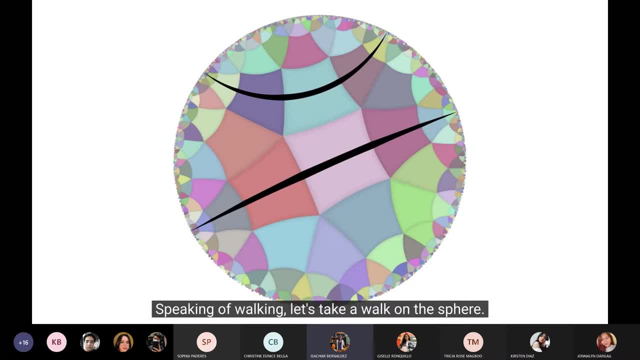 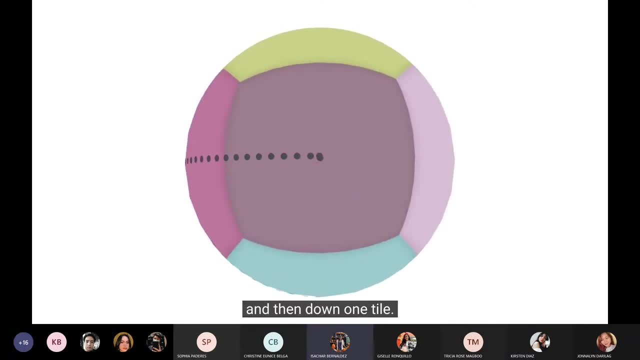 To see it was straight the whole time. Speaking of walking, let's take a walk on the sphere. Let's walk up one tile, right one tile, and then down one tile. We're back where we started And we just walked around a triangle with three right angles. 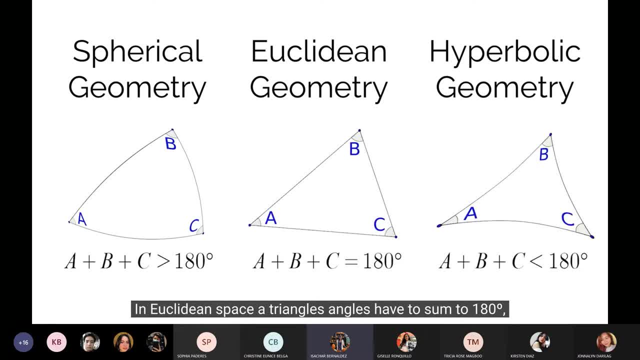 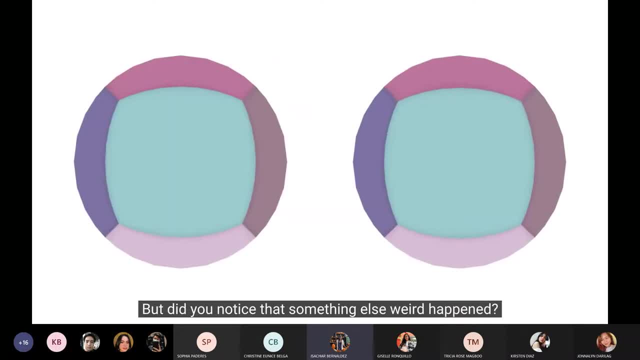 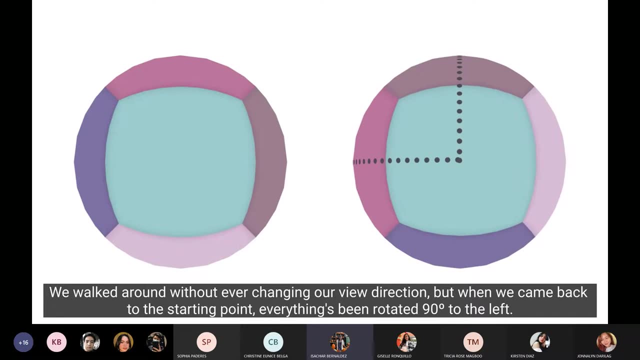 In Euclidean space a triangle's angles have to sum to 180 degrees, But in spherical space it's always larger. But did you notice that something else weird happened? We walked around without ever changing our view direction, But when we came back to the starting point, everything's been rotated 90 degrees to the left. 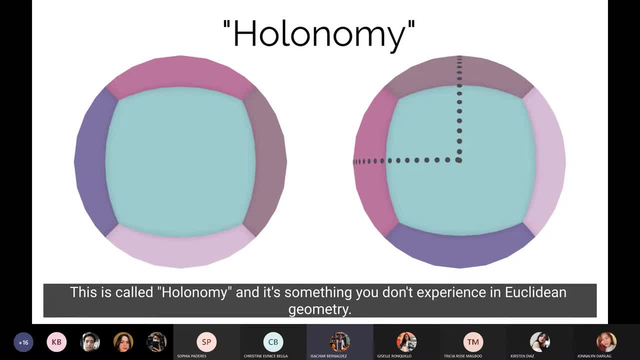 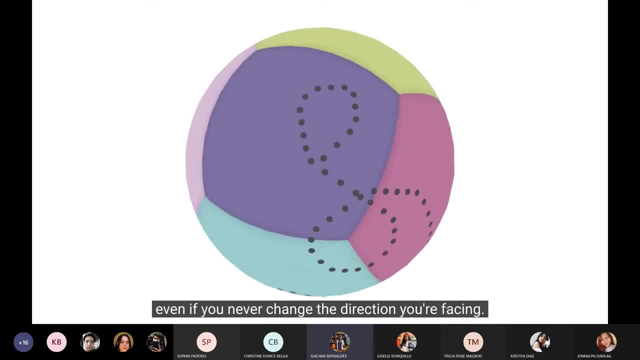 This is called holonomy, and it's something you don't experience in Euclidean geometry. Basically, as you move around the space, you accumulate extra rotation, Even if you never change the direction you're facing. So take a guess what happens on a hyperbolic walk. 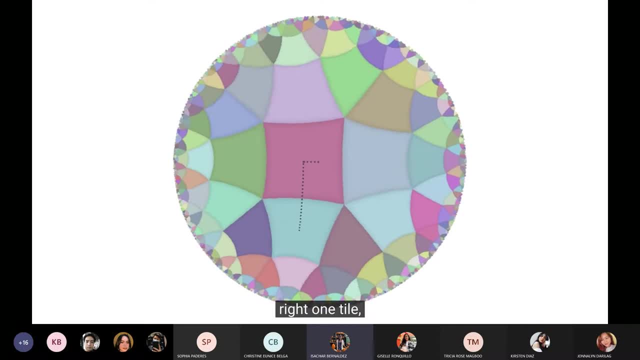 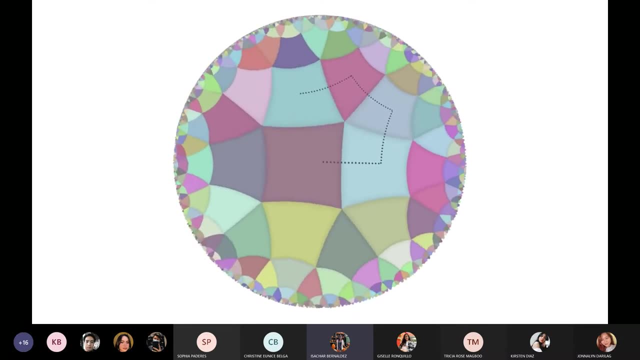 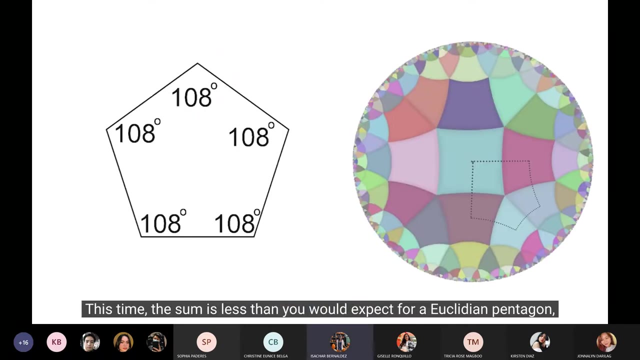 We'll walk up one tile Right, one tile, Down one tile, Left, one tile And finally up one more time. Now we've walked on a pentagon with five right angles. This time the sum is less than you would expect for a Euclidean pentagon. 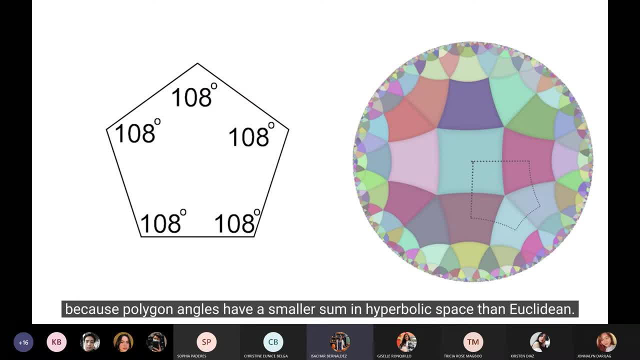 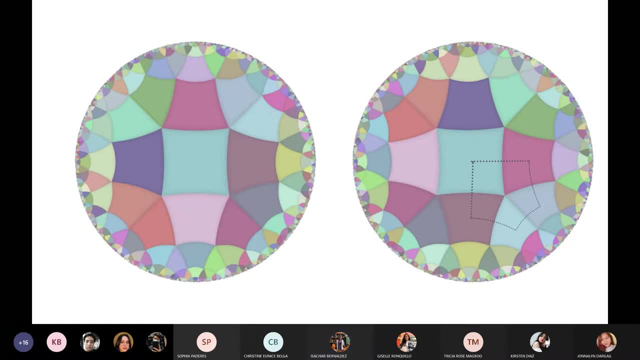 because polygon angles have a smaller sum in hyperbolic space than Euclidean And we have the same holonomy effect, but this time rotated in the opposite direction. One last effect I want to talk about is a physical one. In the real world, objects are made up of smaller particles. 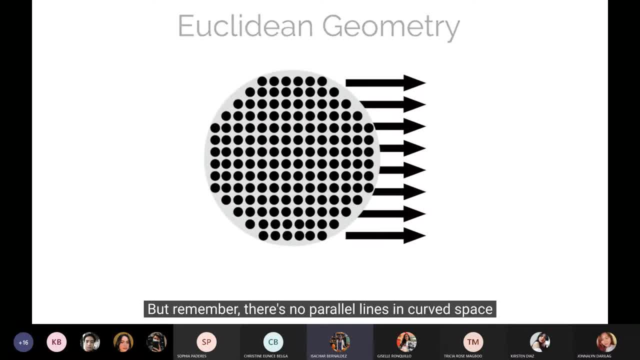 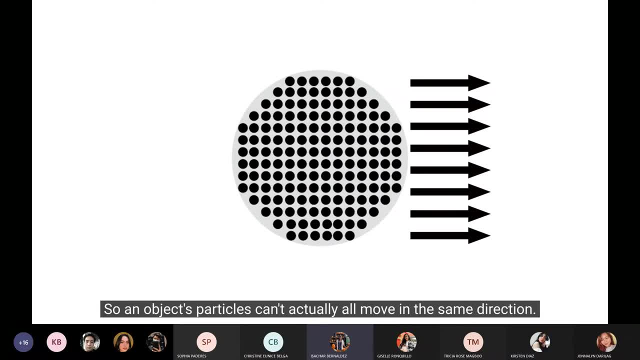 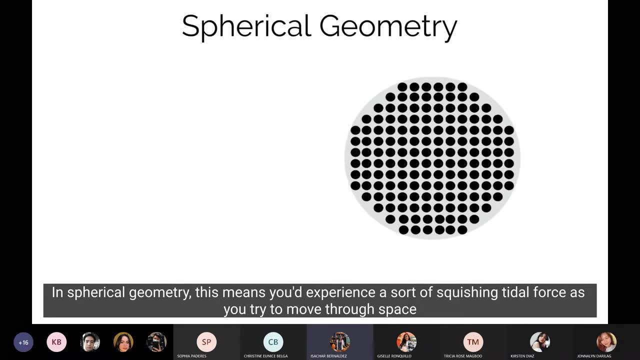 And when an object moves, all of its particles move as well. But remember there's no parallel lines in curved space, So an object's particles can't actually all move in the same direction. In spherical geometry this means you'd experience a sort of squishing tidal force as you try to move through space. 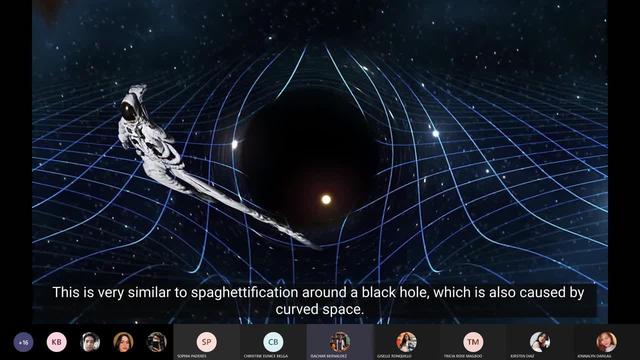 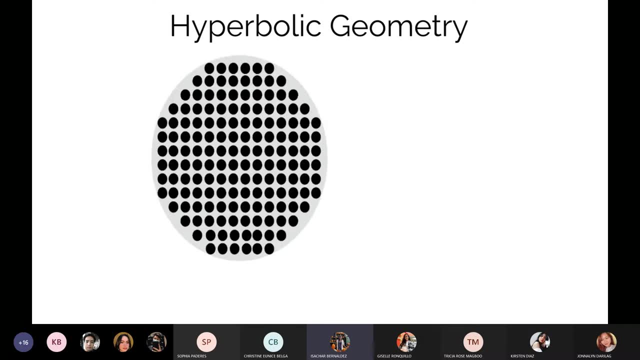 This is very similar to spaghettification around a black hole, which is also caused by curved space And in hyperbolic space. objects experience a stretching tidal force as they move. With enough speed and curvature, hitting a hyperbolic baseball could actually rip it apart. 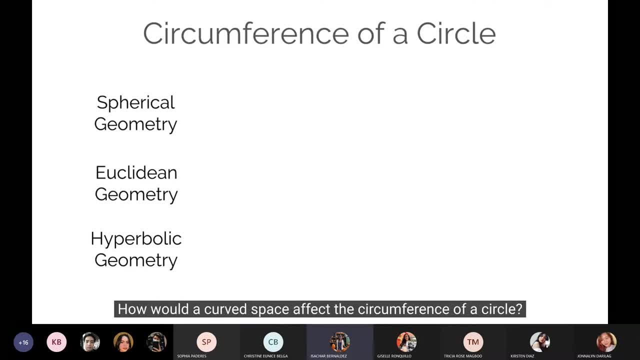 Okay, let's switch over to some formulas. How would a curved space affect the circumference of a circle? It's 2 pi r in Euclidean space, but it's pi sine r in spherical space. It should kind of make sense why this is true. 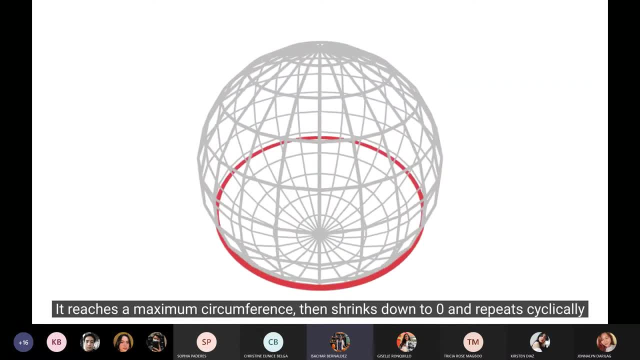 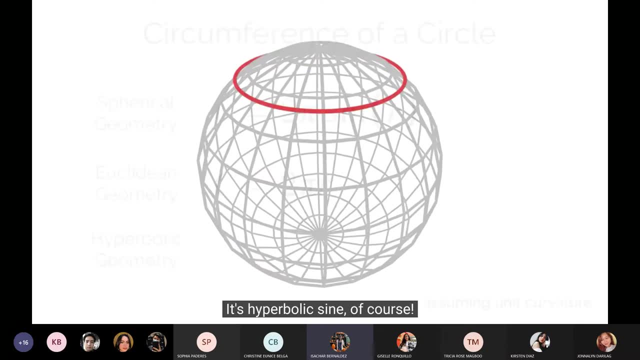 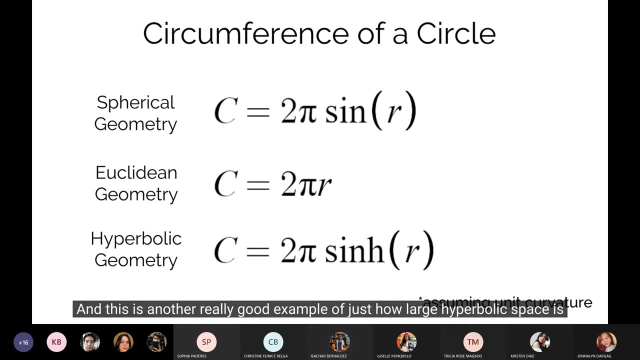 As the radius gets larger, it reaches a maximum circumference. It then shrinks down to zero and repeats cyclically. Want to guess what the hyperbolic opposite is? It's hyperbolic sine, of course, And this is another really good example of how large a circle is. 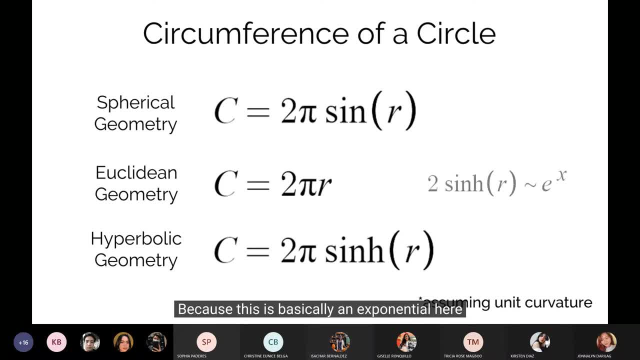 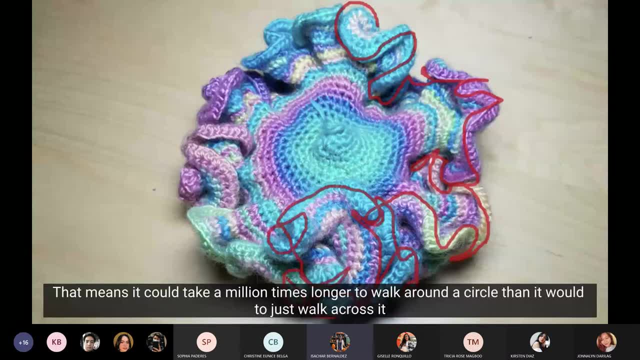 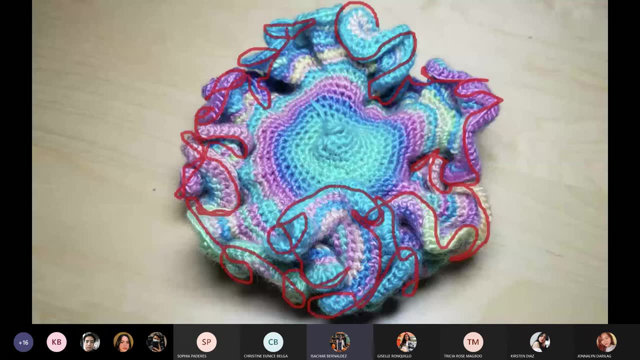 Because this is basically a circle. If you could take a million times longer to walk around a circle, then it would just walk across it. The area of a circle also has similar formulas. Again, area is exceptional for hyperbolic space, But interestingly it grows at the same rate as the circumference, unlike Euclidean space where it grows as the square. 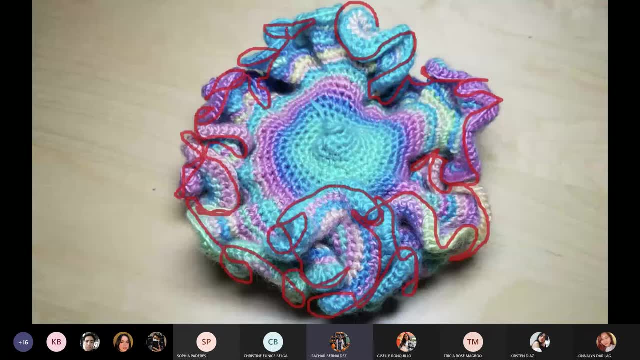 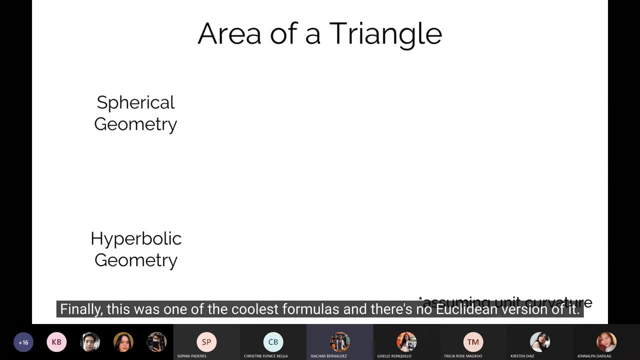 The Pythagorean formula also has really beautiful analogs in curved space. And finally, this was one of the coolest formulas and there's no Euclidean version of it. In a unit curved space, you can find the area of any triangle, given only its angles. 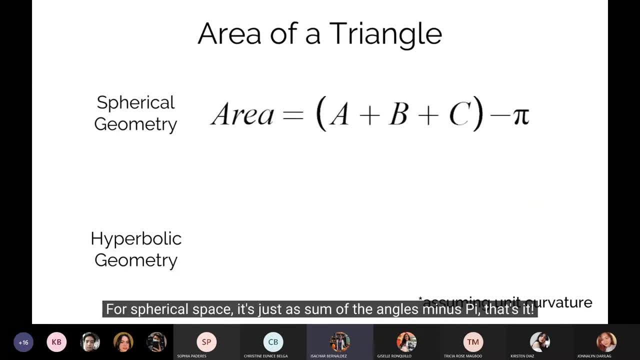 And the formula is so simple. For spherical space it's just the sum of the angles minus pi. That's it. In hyperbolic space, it's pi minus the sum of the angles. Isn't that neat? And there's a good insight from this formula. 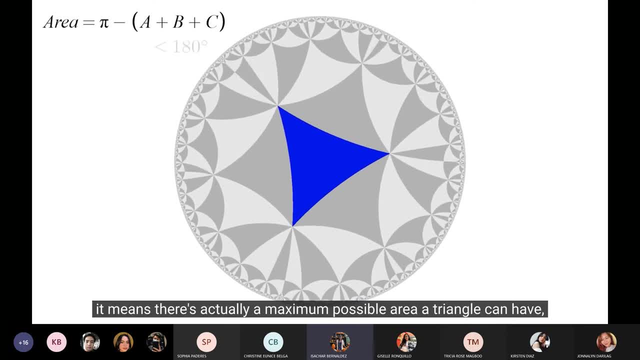 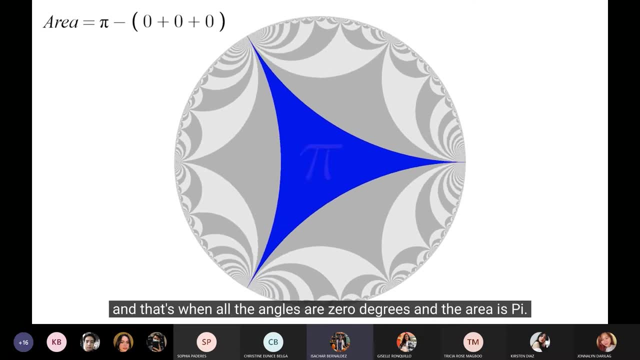 Since the sum is always less than 180 degrees. in hyperbolic space it means there's actually a maximum possible area a triangle can have, And that's when all the angles are zero degrees and the area is pi. It happens because all lines eventually diverge. 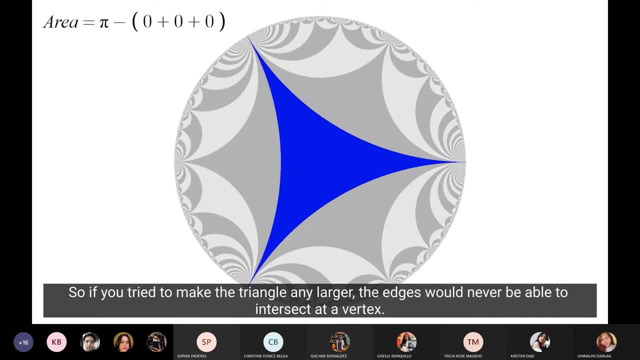 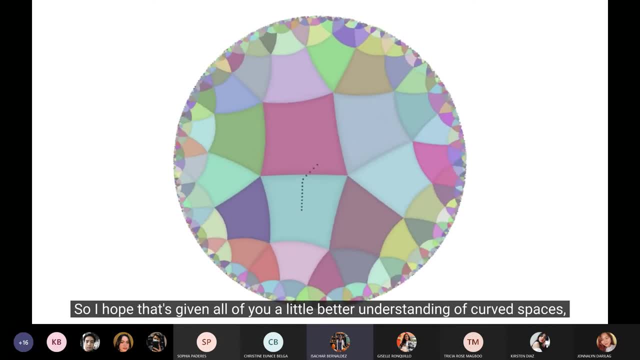 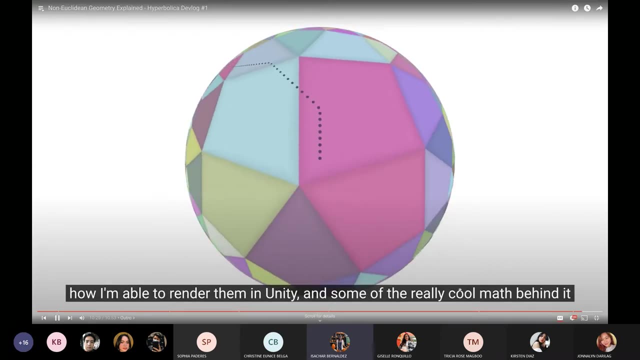 So if you tried to make the triangle any larger, the edges would never be able to intersect at a vertex, So I hope that's given all of you a little better understanding of curved spaces. In the next video I'm going to talk more about three-dimensional spaces, how I'm able to render them in Unity and some of the really cool math behind it. 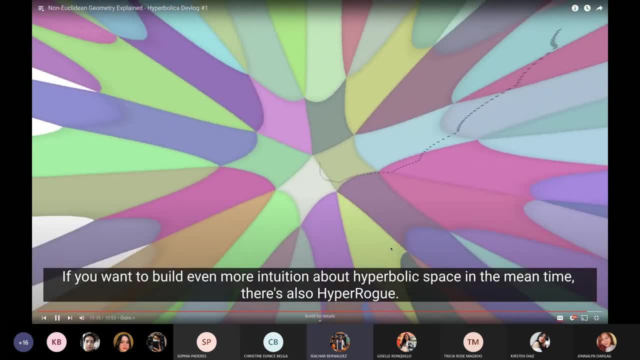 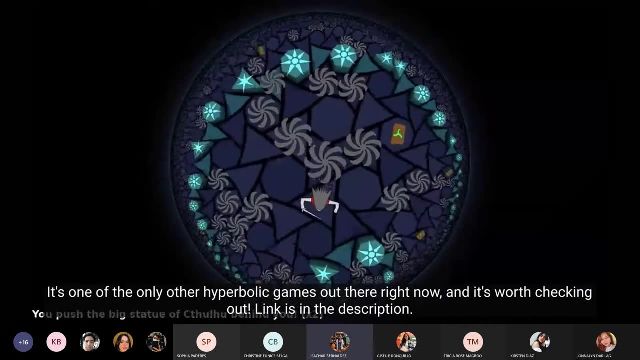 If you want to build even more intuition about hyperbolic space. in the meantime, there's also Hyper Rogue. It's one of the only other hyperbolic games out there right now And it's worth checking out. The link is in the description. 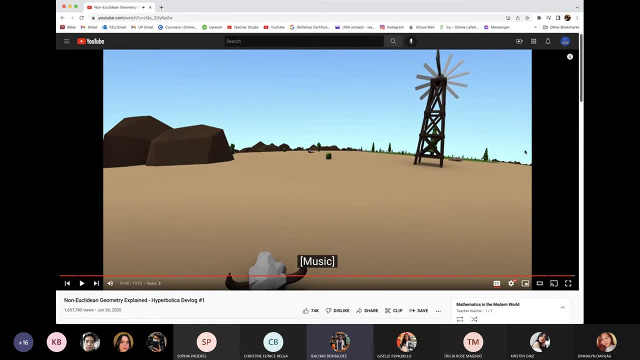 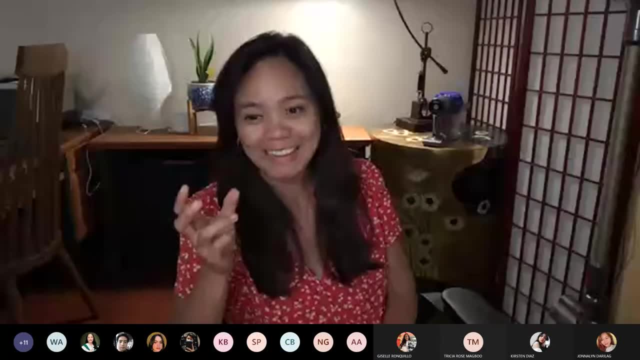 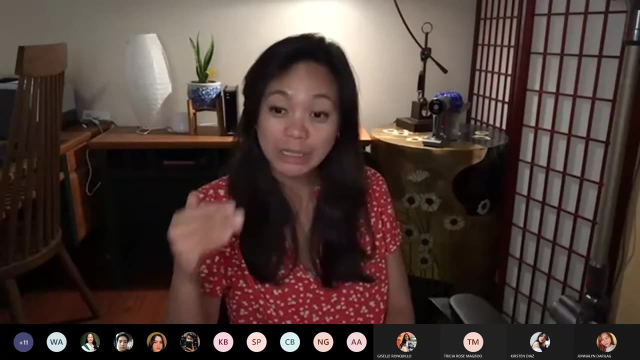 So thanks for coming on this journey and stay hyperbolic There. So we got it. We made a video about it. So that is that we're more familiar with the Euclidean. The Euclidean is just an x and y axis. 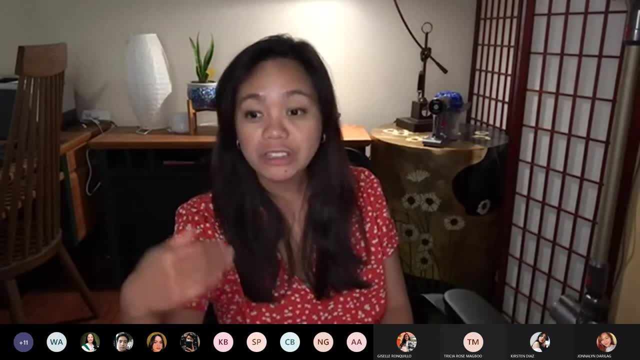 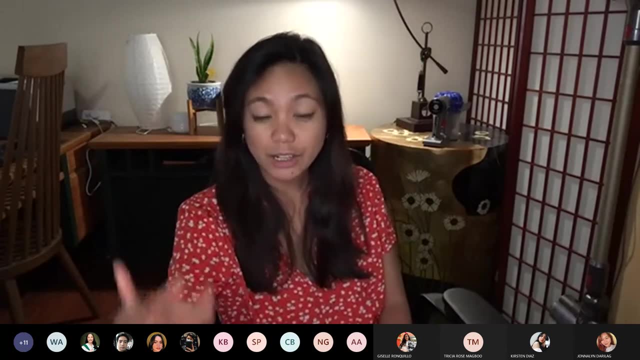 We can also use an x and y z axis. But when it comes to other types of geometry, when it comes to roundness, what we call that is spherical or elliptic. There's another word for it- It's called elliptic geometry. 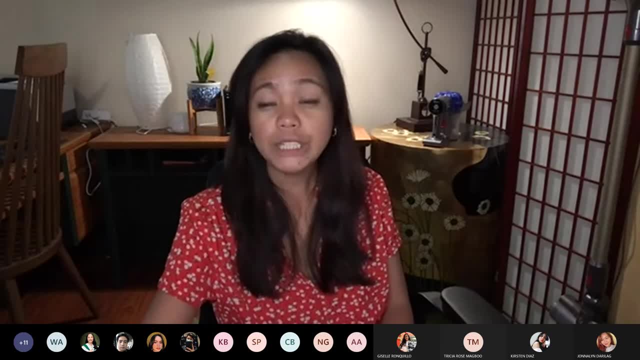 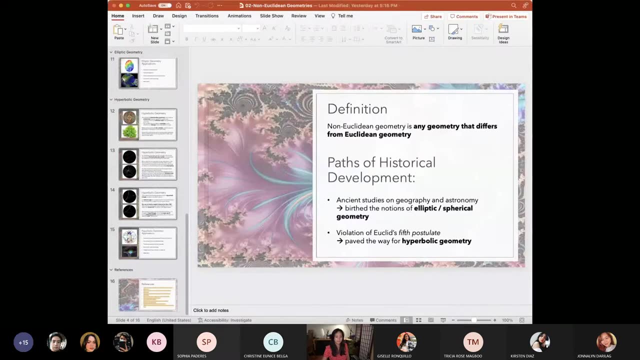 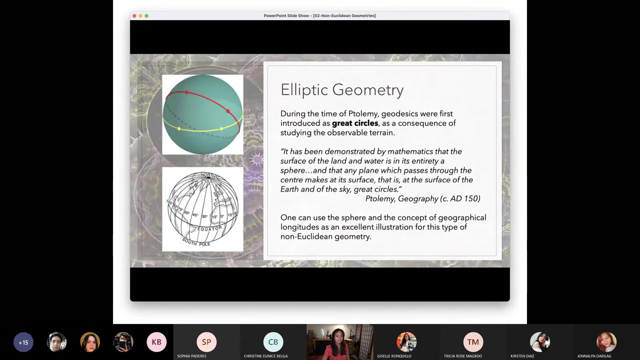 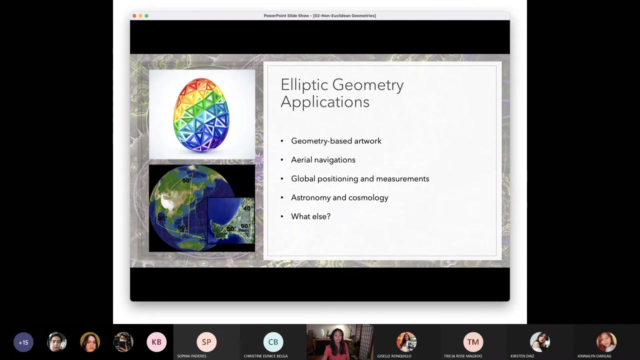 Now, in elliptic geometry, this is what we use, So I'll share our PowerPoint. So, for elliptic geometry, It's more used when it comes to aerial navigation, Like how to position, global positioning and measurements. So, as we discussed earlier, if you noticed, 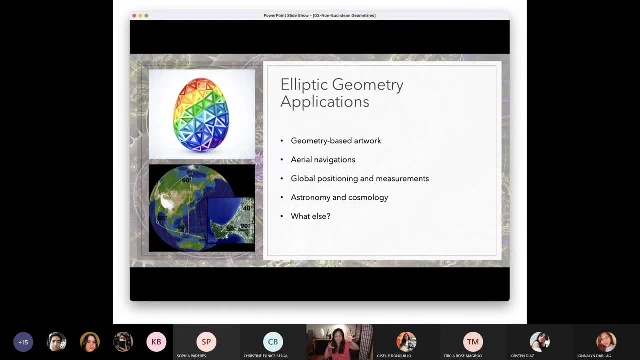 when the map is flat, you'll feel that the Greenland and Africa are the same size. But when you curve them, since they're at the top, when you curve them, we'll know that they're really different in size. So spherical, or what we call the elliptic geometry, has an application in aerial navigation for airplanes. 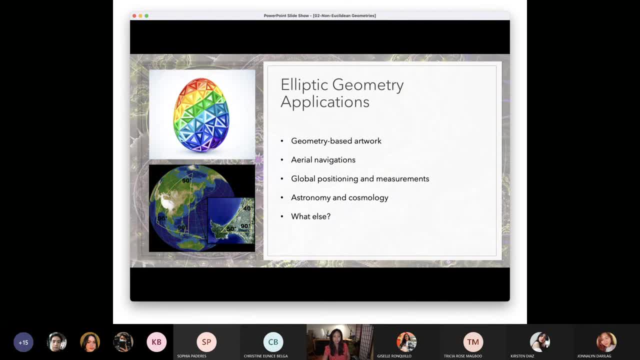 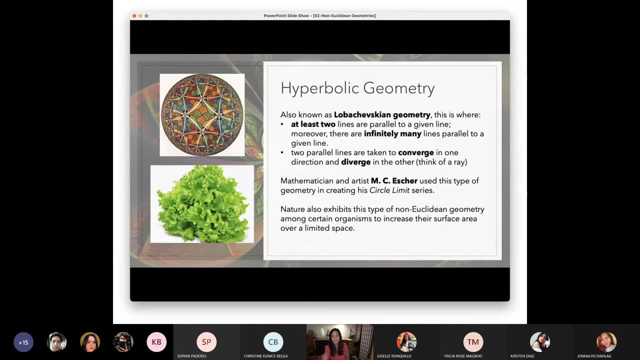 for anything that's moving above the sky: global positioning and measurement, astronomy and cosmology, and art, of course, and other stuff. Now for hyperbolic. hyperbolic is not actually visible in nature, Like, for example, these vegetables. 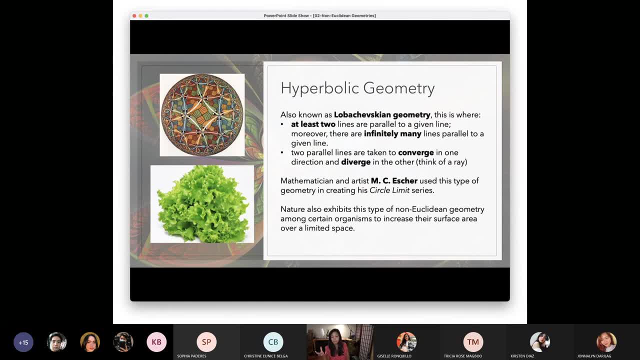 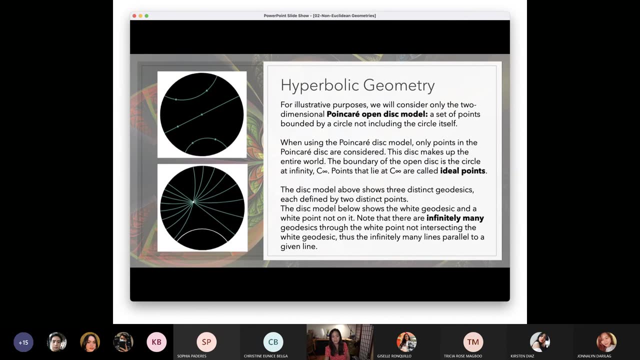 fractals, really beautiful microorganisms. They have these shapes that are not euclidean and not spherical, So we call this the hyperbolic geometry. So in hyperbolic geometry you'll notice that it's used for art, of course.